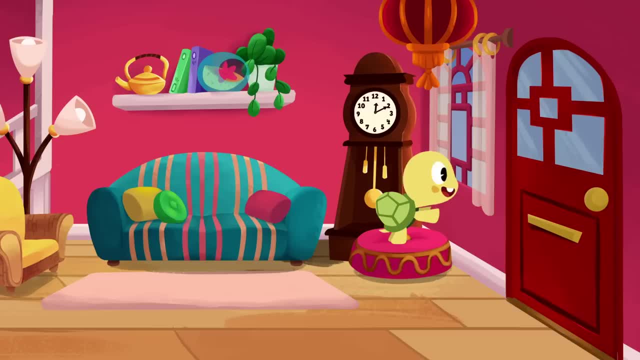 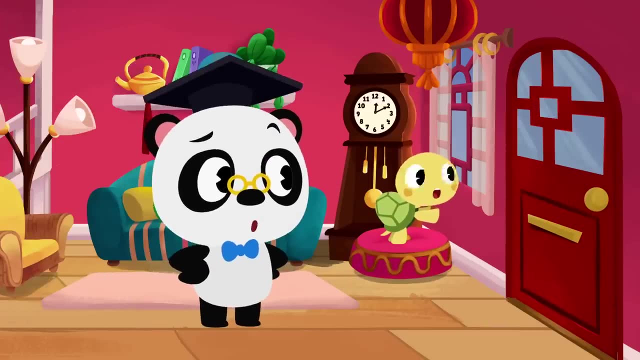 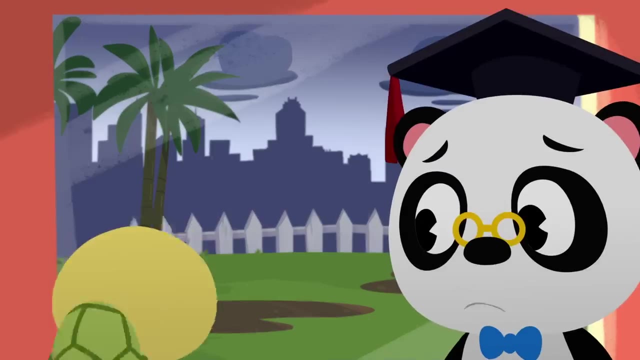 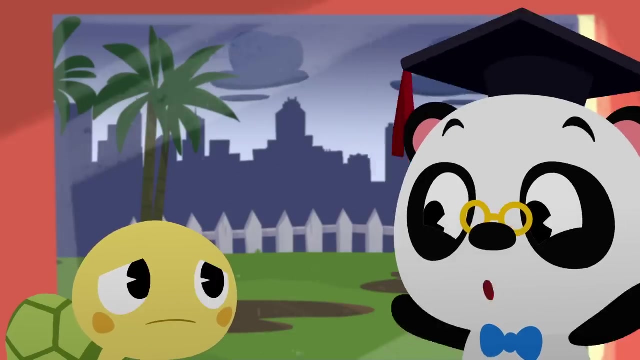 Search for Dr Panda Morning Toto Playtime Outside- Outside- Aw, what a shame We can't play outside in this weather, Toto. Aw, no playtime. No worries, Toto, There's lots of fun things to do inside the house. 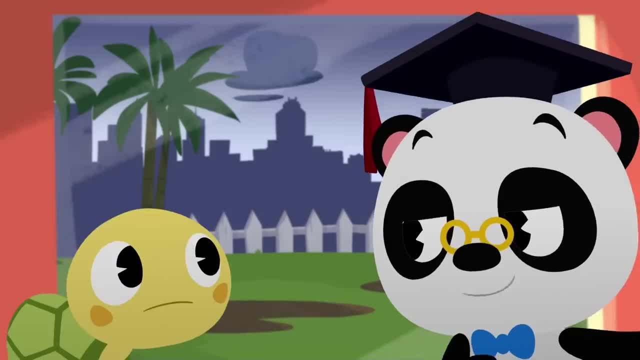 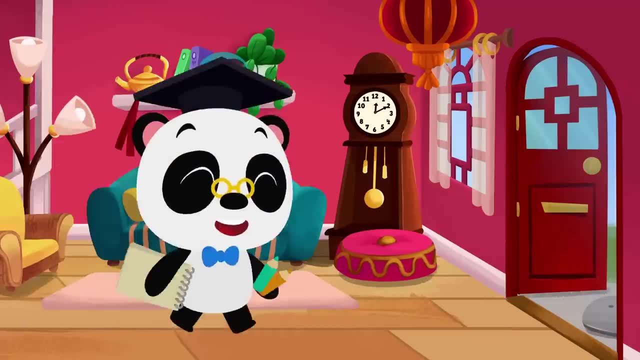 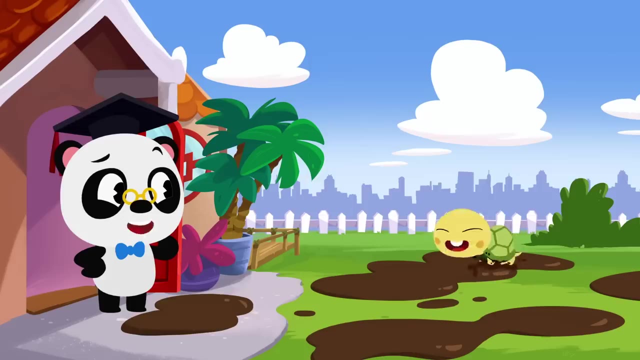 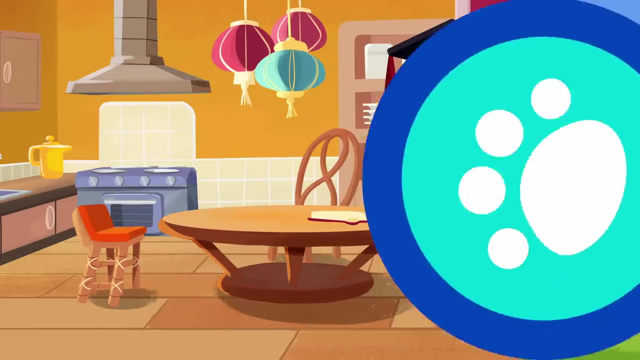 How about some drawing? I'll go and get some paper and pens. Here we go. What shall we draw first? Toto, I guess it stopped raining. Have fun playing in the mud, Toto. Hmm, I wonder if Toto's still playing in the mud. 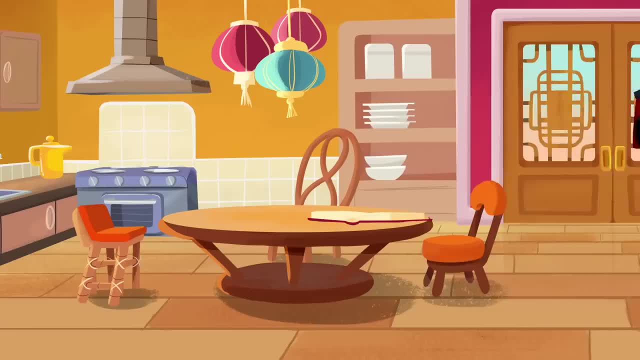 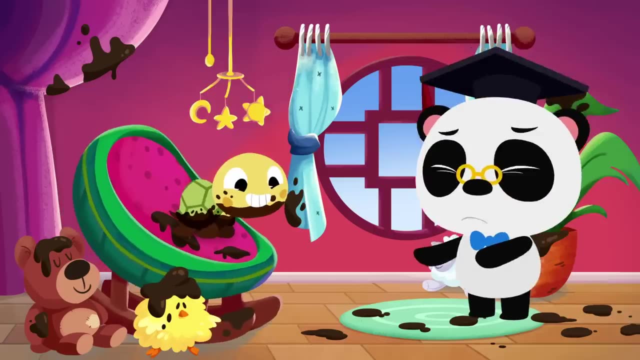 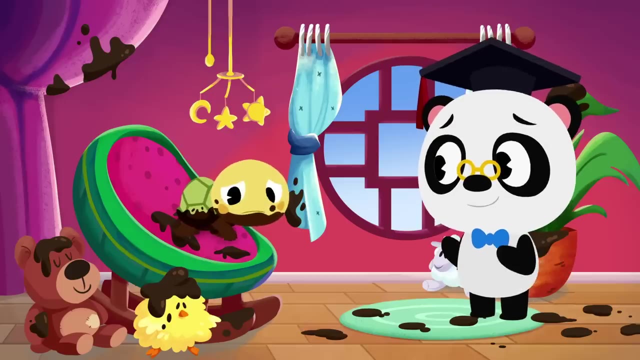 I sure don't. I sure don't want him to walk into the house with his feet alldirty. Toto, what are you doing? You're making everything dirty. Oops, sorry, Aw, no worries, We can clean it up, But first we have to get you clean. 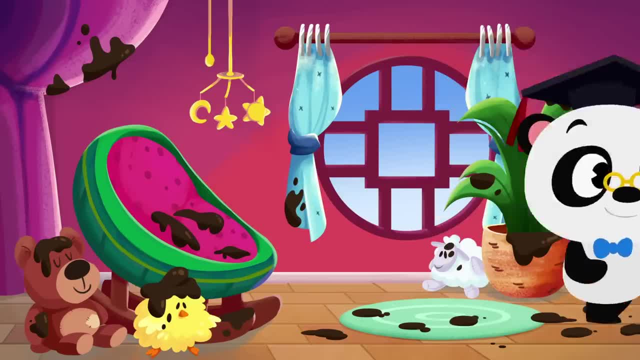 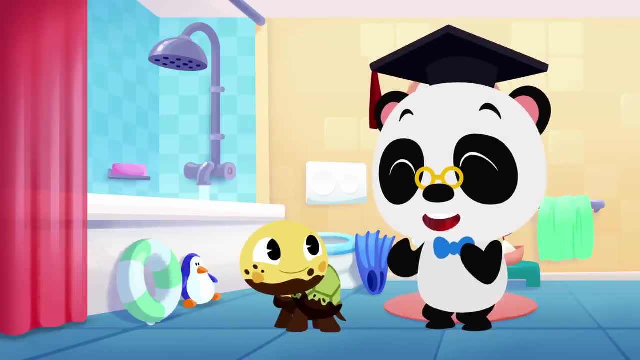 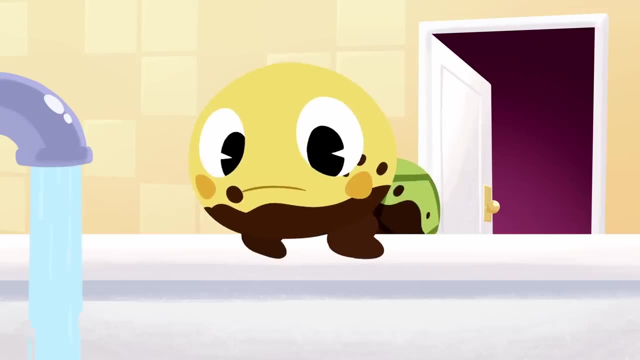 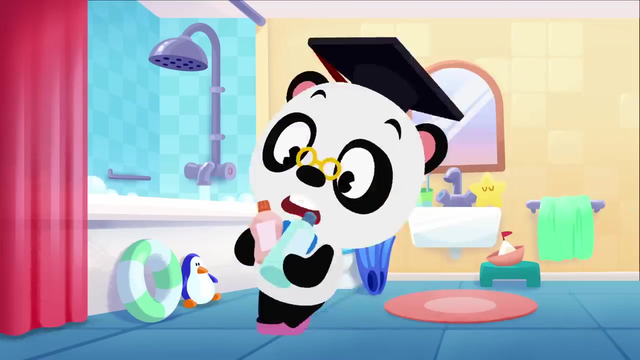 Time for a bath, Bath, Bath. You'll have to wait a bit for the bath to fill up. Toto, I'll go get some bubble bath to make some bubbles. Toto, where are you going? Toto, come back. 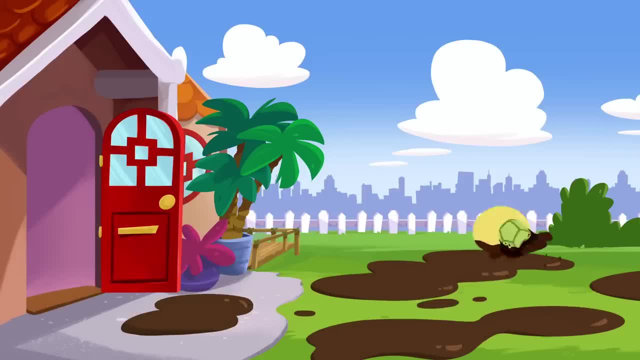 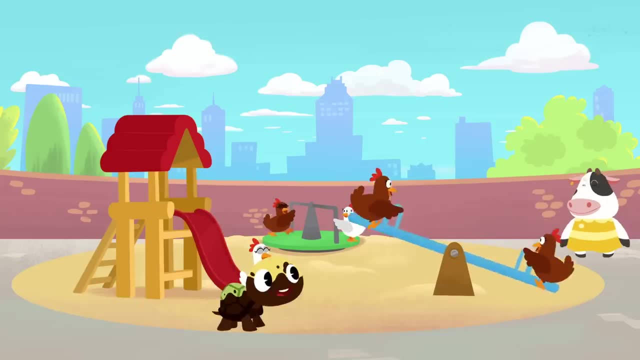 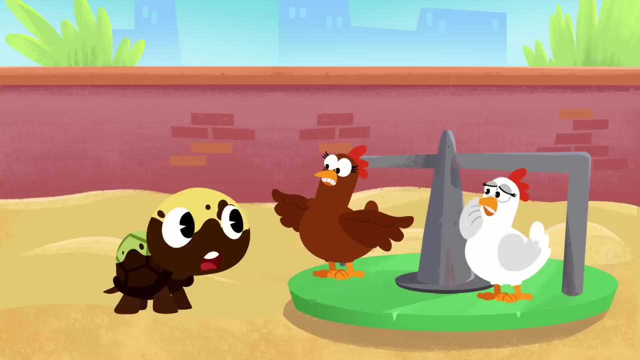 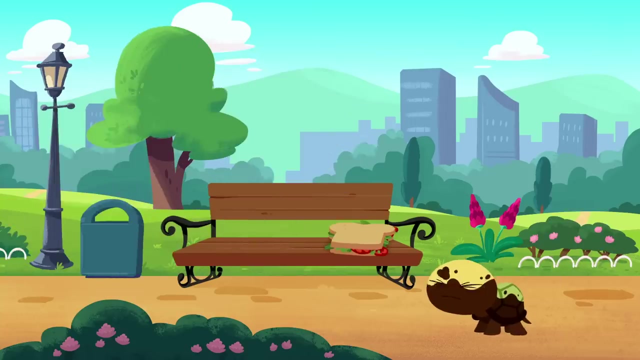 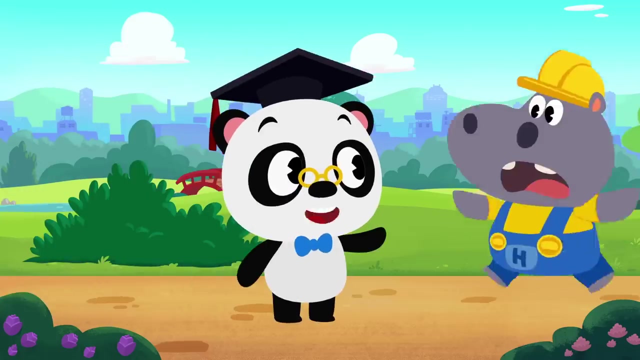 Playtime Outside: Chickens- Playtime Chickens- No, No, playtime. Pooper Playtime- No, playtime Toto, Toto Toto. Hey Hoopa, have you seen Toto Toto? there you are. 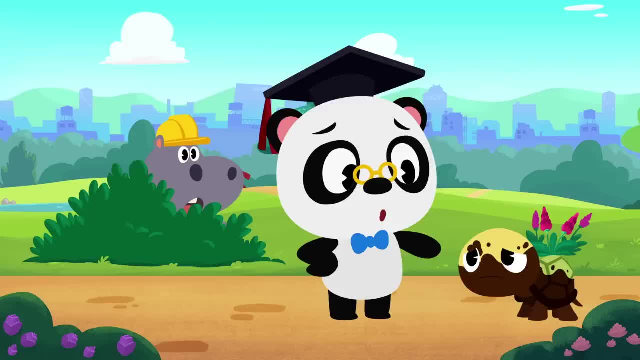 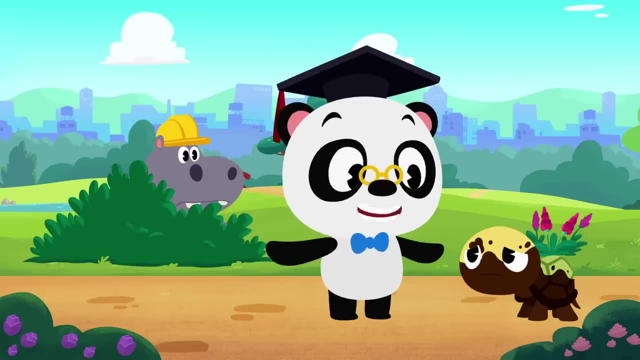 You're so covered in mud I didn't see you. No playtime. Aw, I get it. No one wants to play with you because you're so muddy And Hoopa didn't even recognize you. I bet you're ready for your bath now, aren't you? 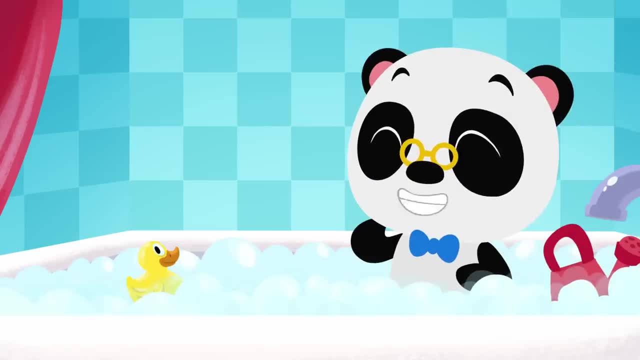 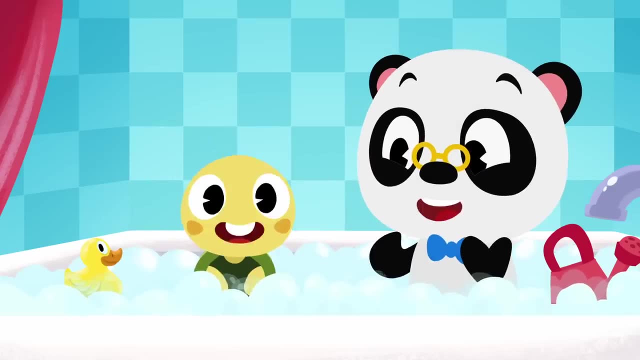 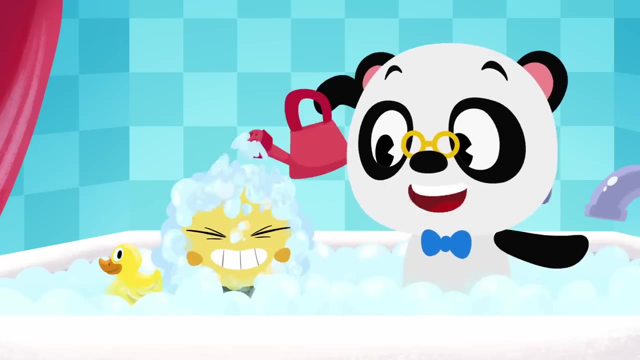 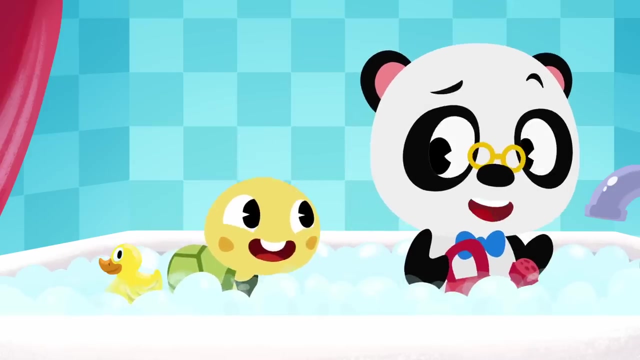 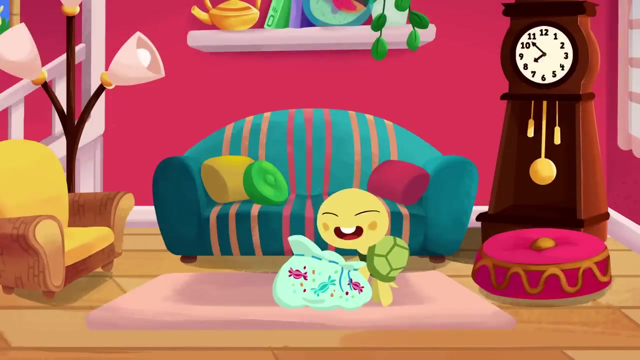 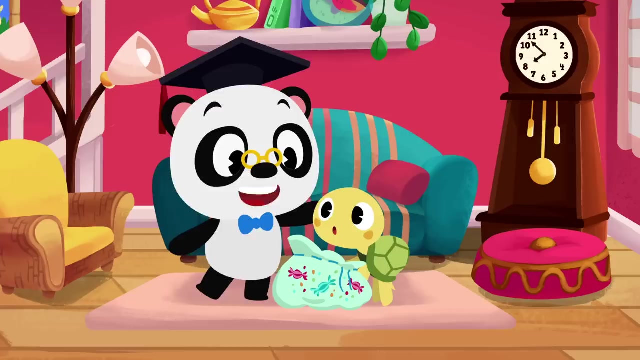 Yeah, Toto, Toto, Whee, Playtime, Bath, Bath, Bubbles. See, Toto, Playing inside can be just as much fun as playing outside. Yeah, Mmm yum, Candy Candy. Nobody should play over there. 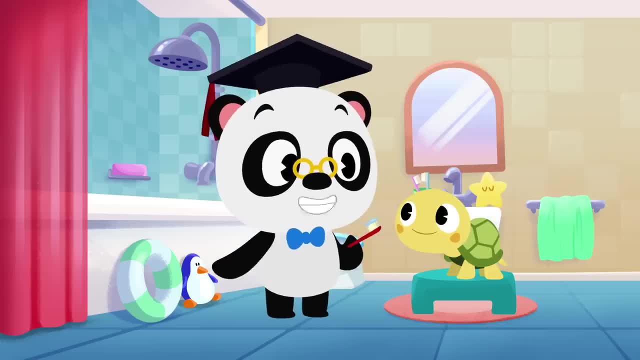 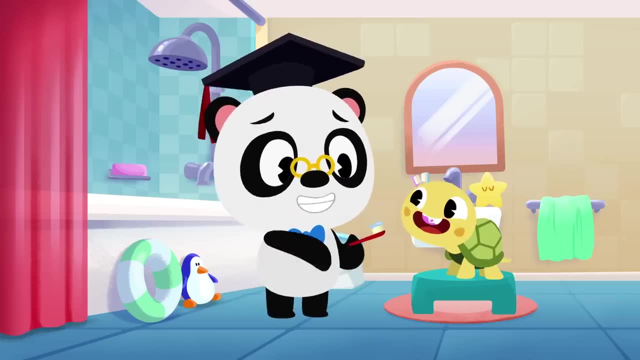 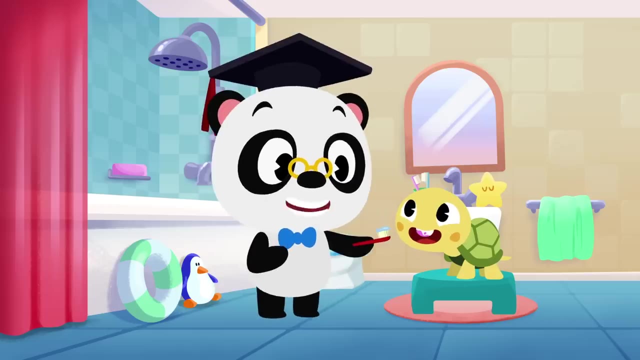 Oh yeah, alright, It's paprika-flavored candy, my favorite, known as Ash. We made this to eat. But stand up, Toto. No more candy. Nevermind, Toto, it's bedtime anyway. Up down and all around. 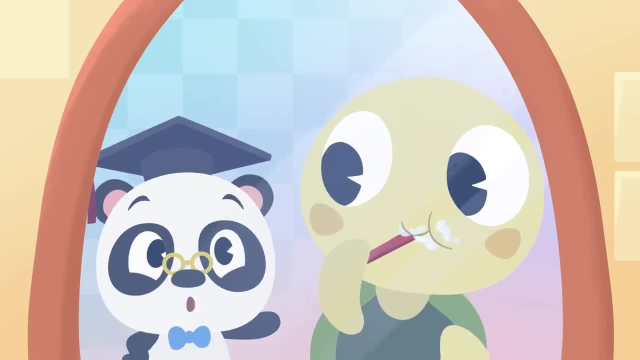 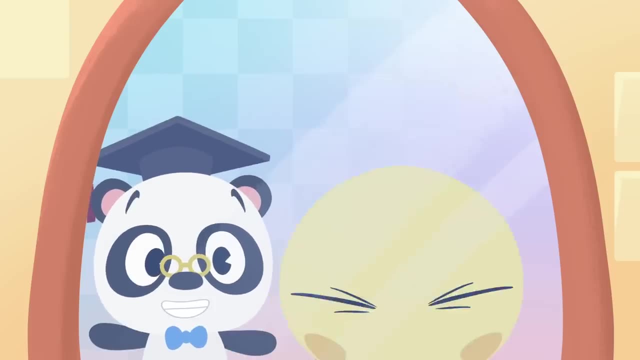 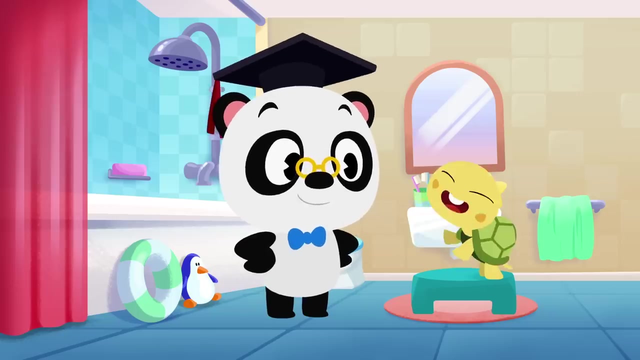 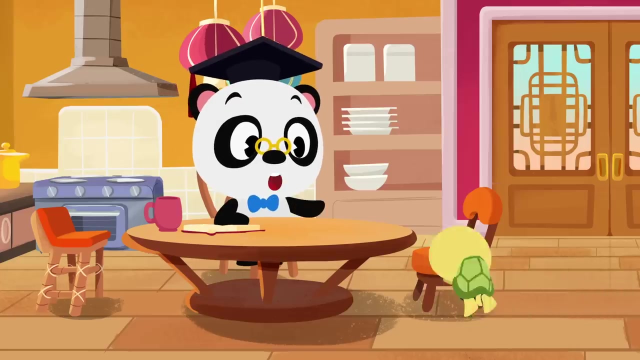 Up down and all around. One last time: Up down and all around. Now rinse- Awesome, Your teeth are sparkling clean again, Toto, Yay, Good morning Toto. Oh, what's wrong Toto? 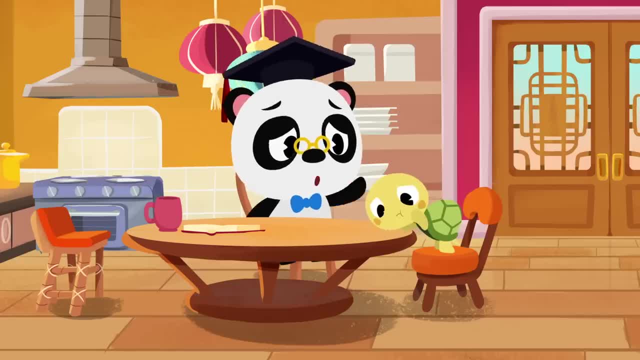 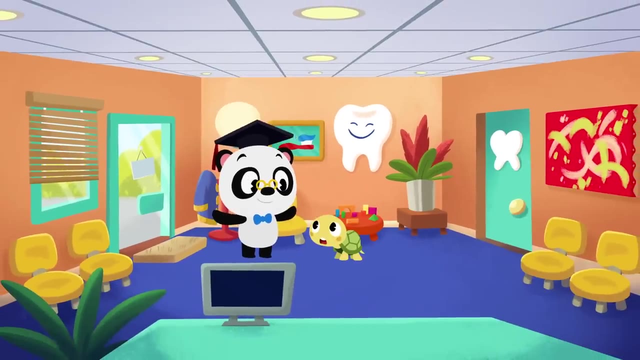 Oh, Oh, your tooth hurts. Hmm, maybe you ate too much candy. Too much candy is bad for your teeth. No worries, Toto, I know who can help The dentist. Huh, The dentist is a special doctor for your teeth. 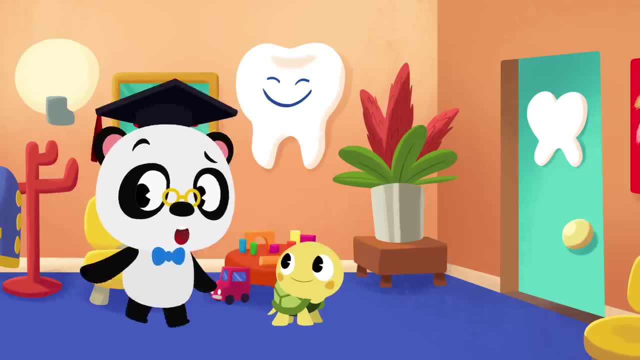 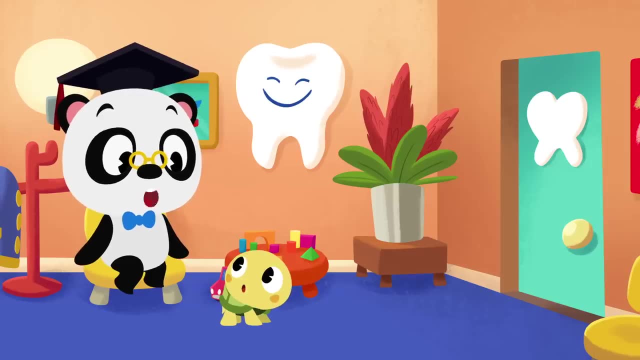 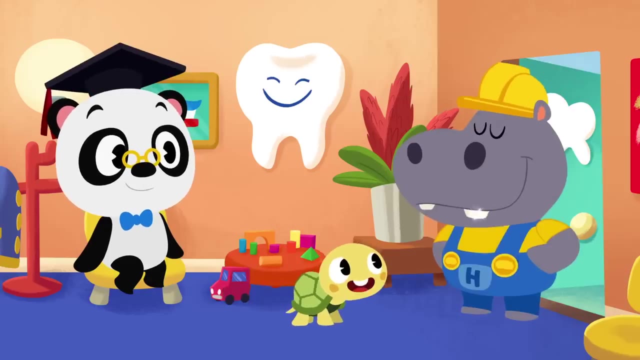 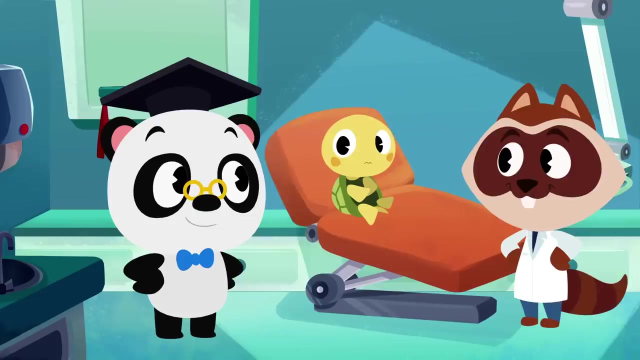 He can take the pain away and tell us what's wrong with your teeth. Oh really, Those noises are just the dentist's tools, Toto, They make all kinds of funny noises. Nothing to be worried about: Richie here is going to have a look at your teeth. 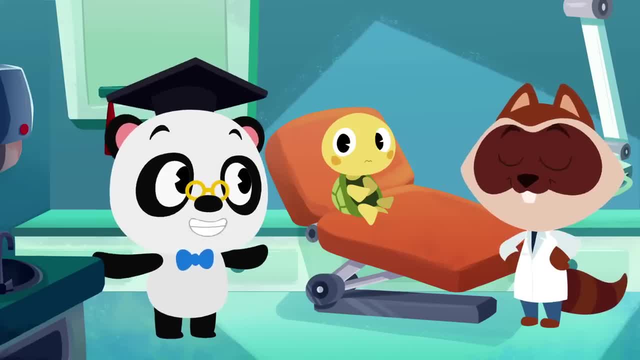 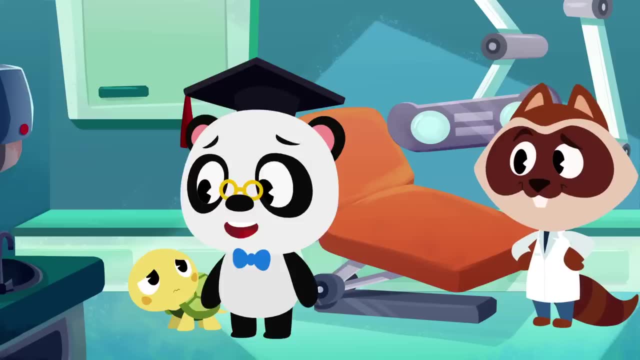 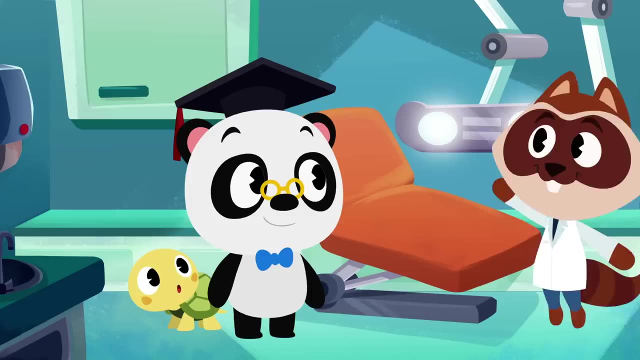 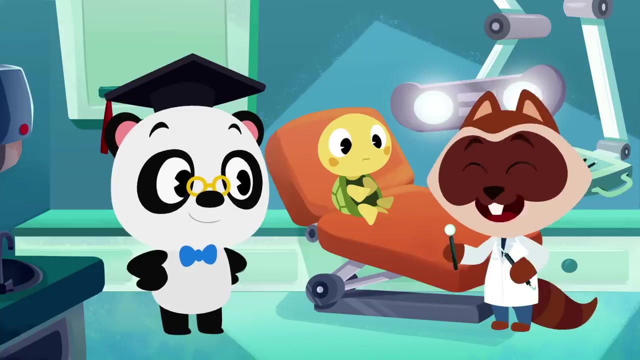 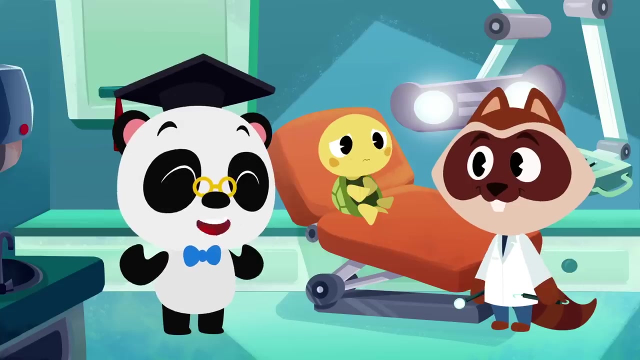 You need to open your mouth as wide as you can. Errrrr, Toto, it's only a light See. Hmm, Oh, That's called a dental probe and mirror. They help, Richie, see the hard-to-reach areas in your mouth. 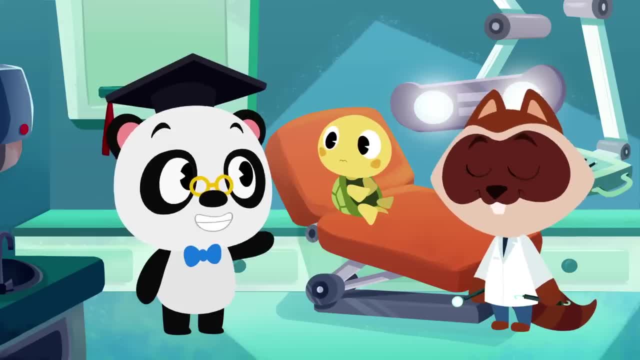 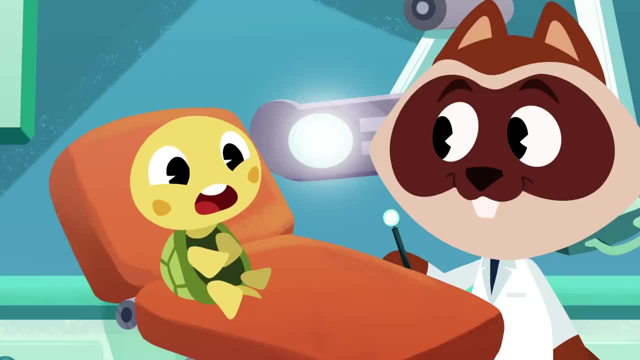 They don't hurt. Look, I'll show you. See, All good, Errrrr, That's only an x-ray machine, Toto. It takes really awesome pictures of the inside of your mouth. Errrrr, There, All done. 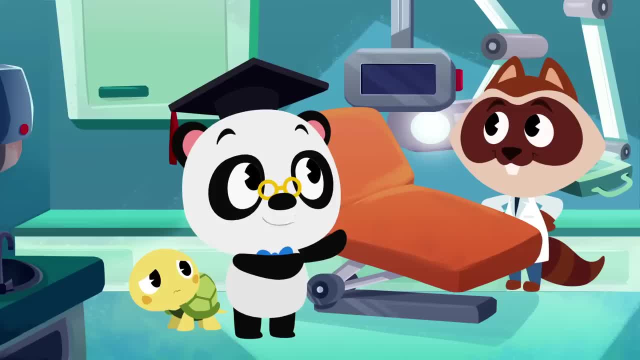 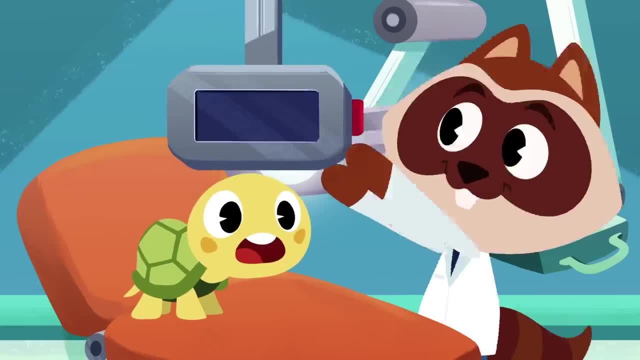 Now let's see what you can do with your teeth. Toto, I'll show you how to do it. I'll show you how to do it with my teeth. I'll show you how to do it with my teeth. I'll show you how to do it with my teeth. 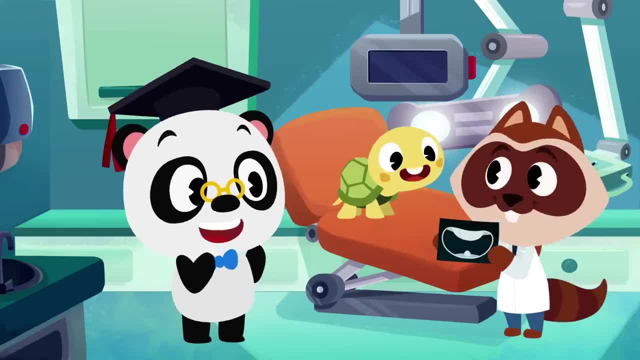 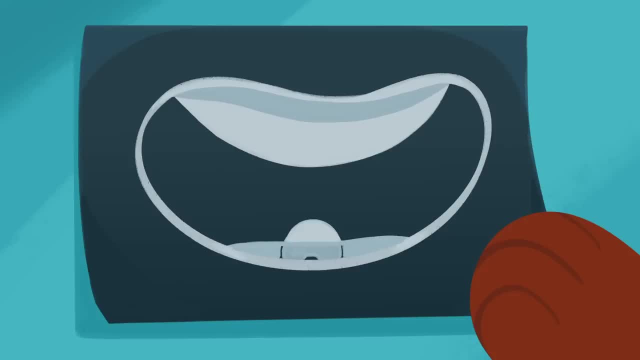 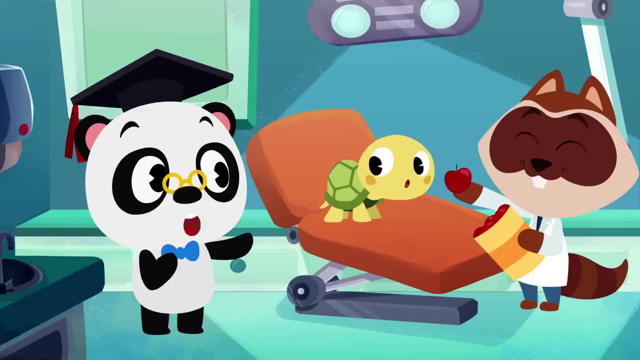 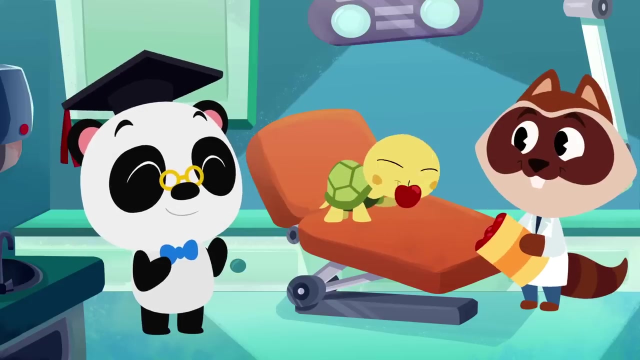 I'll show you. Errrrrr, Oh, I see You have a new tooth growing, Toto. That's why it was hurting Candy. Those are apples, Toto, The best kind of candy you can eat- Yummy apples. 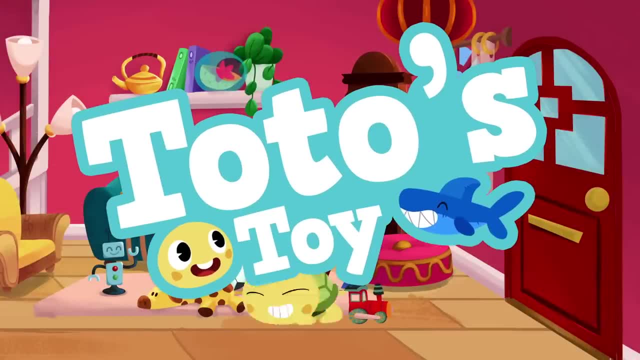 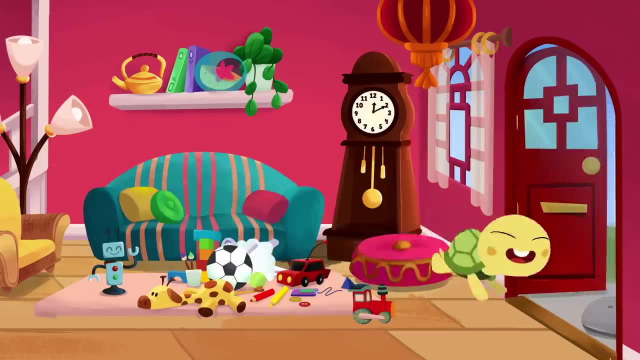 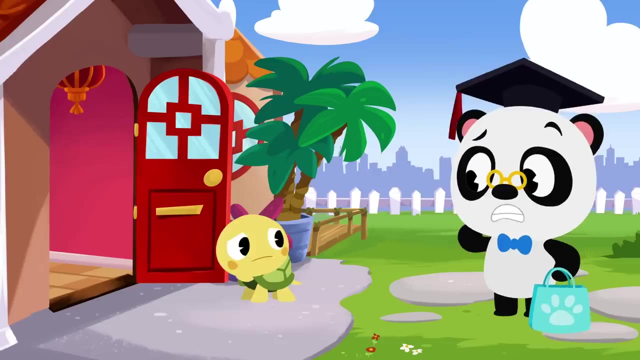 Hey, Oh, a strawberry. Um Ah, Ah. Hey, Toto, it's time to go and get our groceries at the supermarket. Yeah, Huh, What's the matter, Toto, Shark, Shark, Oh, you forgot to bring your favorite toy with you. 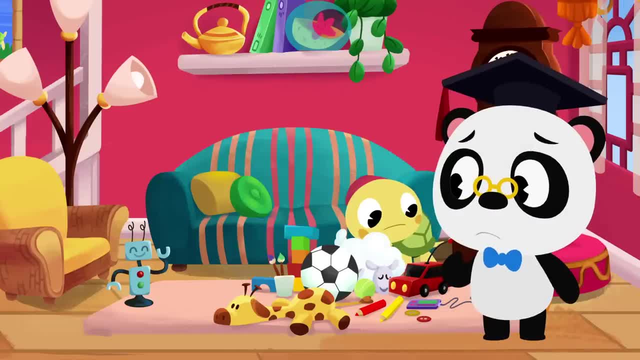 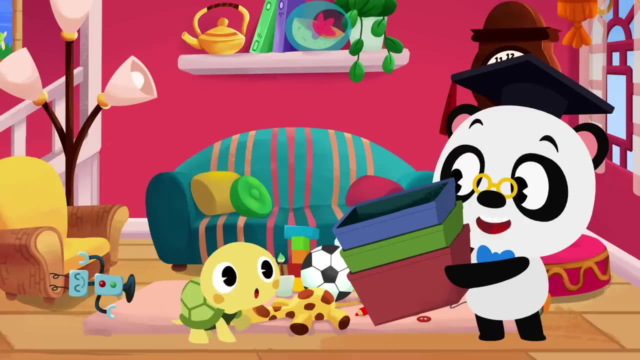 No worries, Let's go get it. Hmm, I don't see your shark anywhere, But there are a lot of toys lying around. No worries, Toto, I've got an idea. Why don't we sort out all your toys and put them in these boxes? 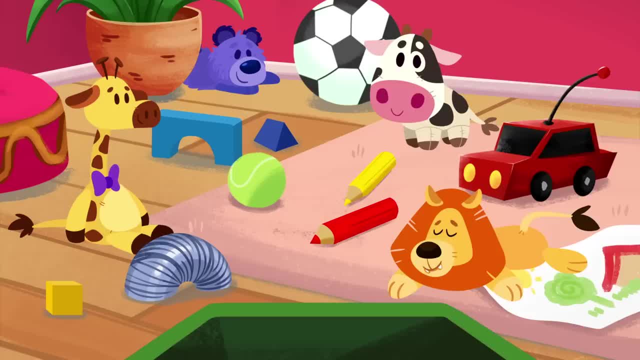 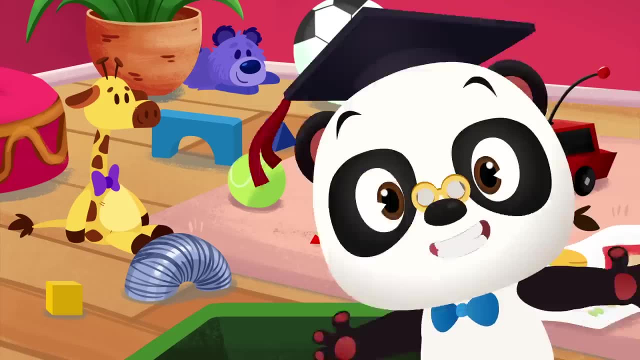 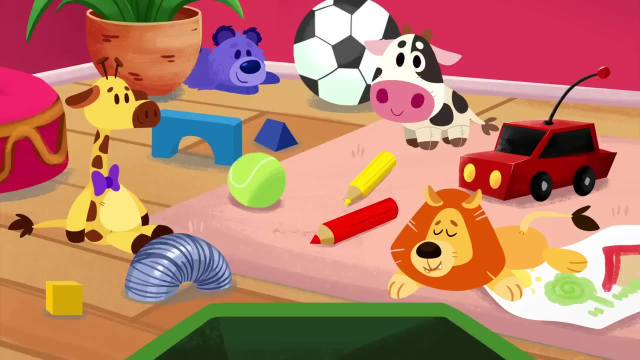 That'll make it easier to find the toys you want to play with. A shark is an animal. Let's try to find all the toy animals and put them in this green box. Can you help Toto spot all the animal toys? Yep, that's right. 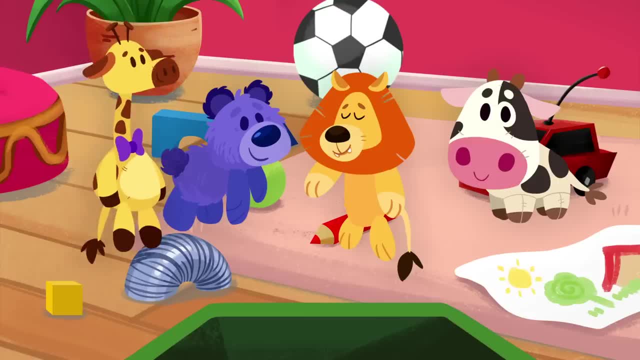 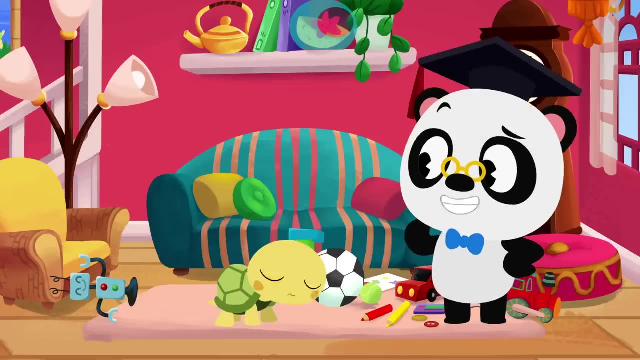 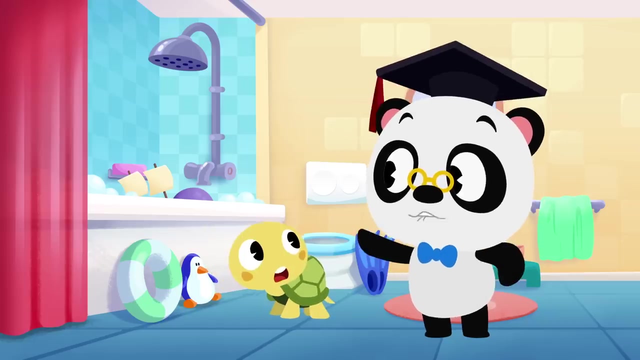 These are all animal toys, Hmm, but I don't see the shark anywhere. Where was the last place you played with your toy shark, Toto? Huh, Buff, Buff. Let's see if your shark is in the bathtub. Yeah, 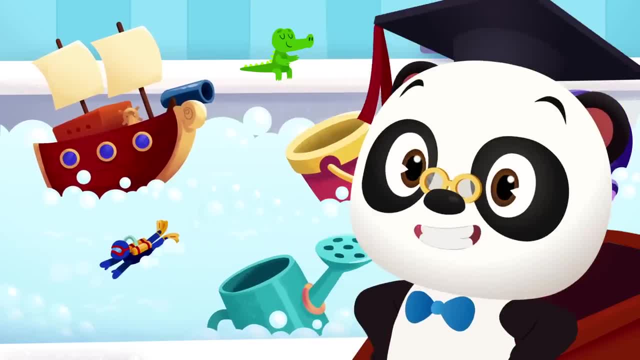 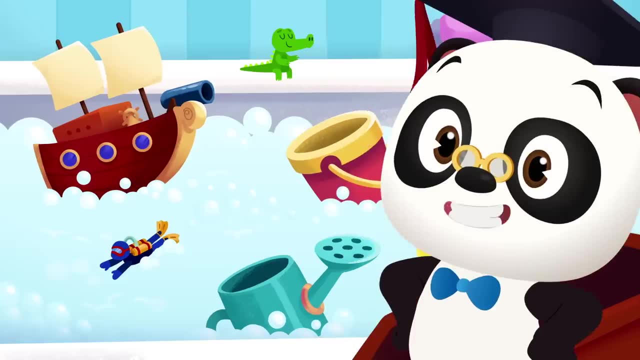 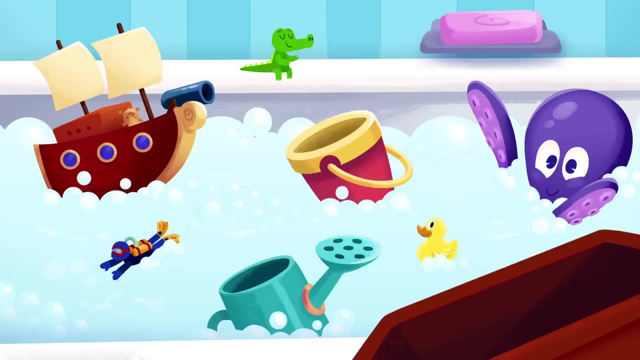 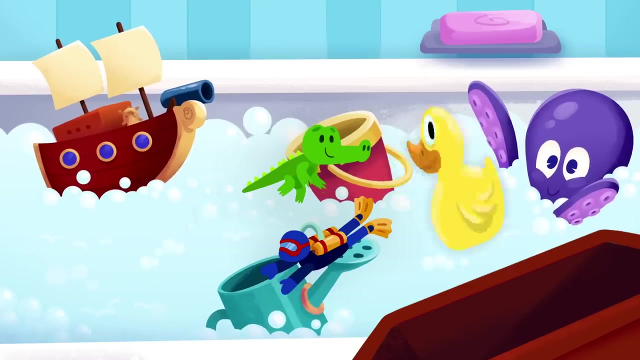 Buff, The small toys belong to Toto And the big toys belong to me. The shark is a small toy. Can you help Toto spot all the small toys in the tub? That's right, These toys are all small. Now only the big toys are left. 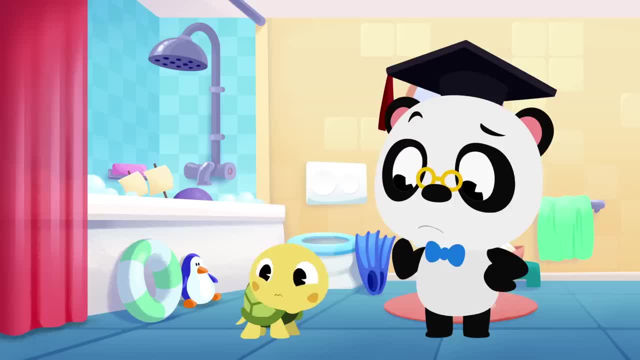 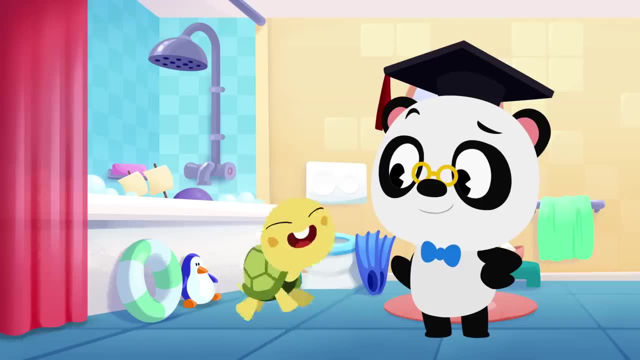 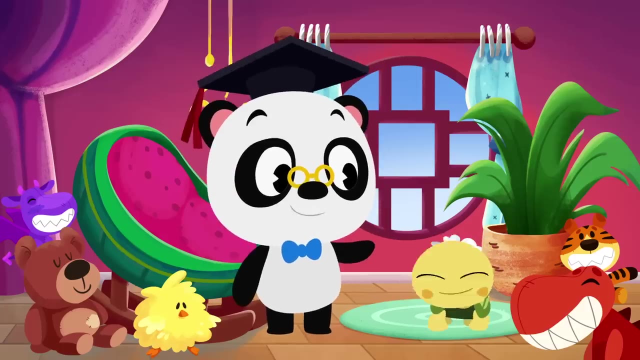 Ah, So where could your toy shark be? Toto, do you remember where you took your shark after you played with it? in the bathtub Bed, Bed? Look at all these stuffed toys. Let's see. Your shark also has sharp teeth. 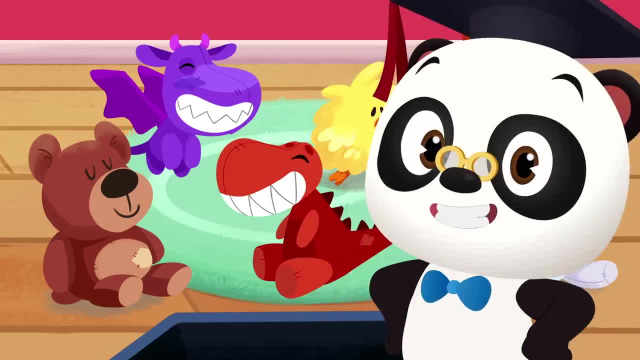 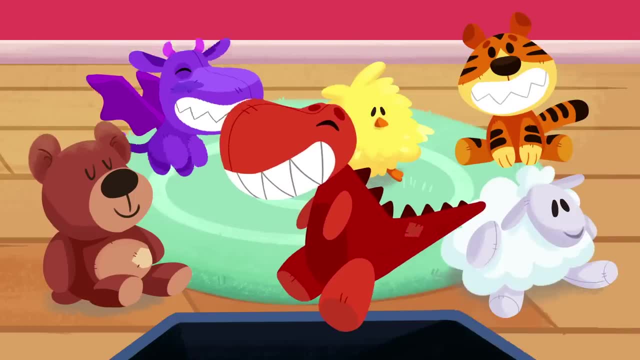 So let's try and find all the toys with sharp teeth. Can you help Toto spot them? Yeah, Yeah, Yeah, Yeah, Yeah, Dinosaur, Dinosaur, Dragon, Dragon, Tiger, Tiger, Tiger. Yeah, You got it. 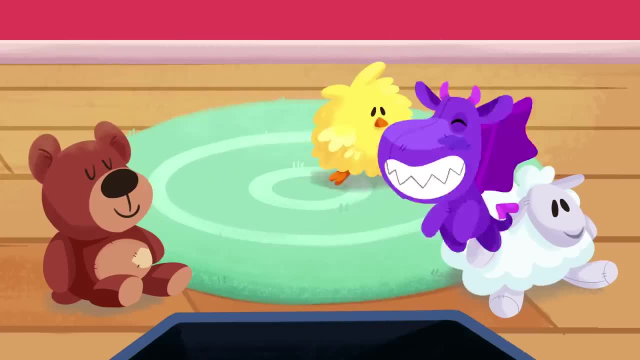 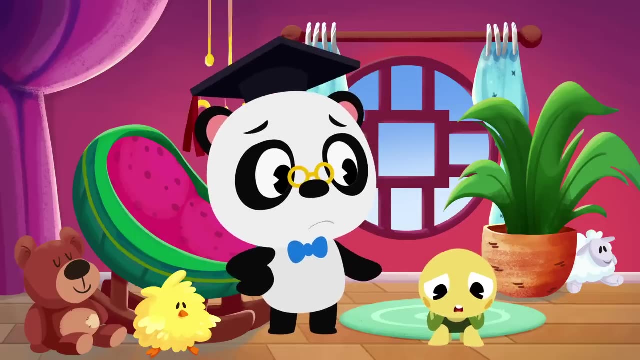 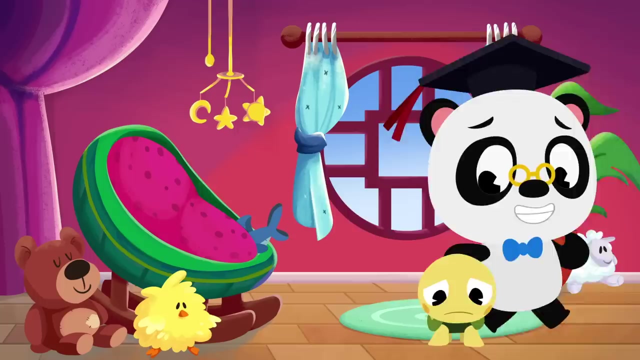 All these toys have sharp teeth. Ah, But we still haven't found your toy shark. I'm sorry, Toto, It's getting late. We're going to have to leave without your shark or the supermarket will be closed. Nom, nom, nom. 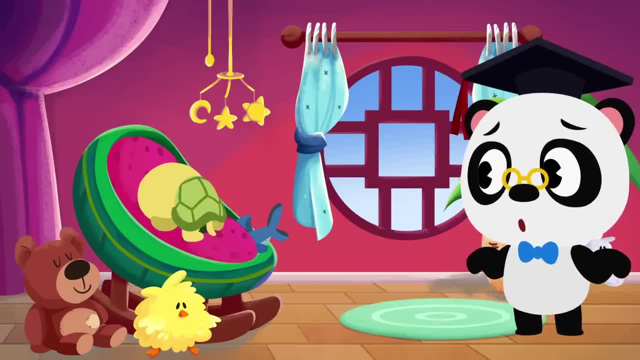 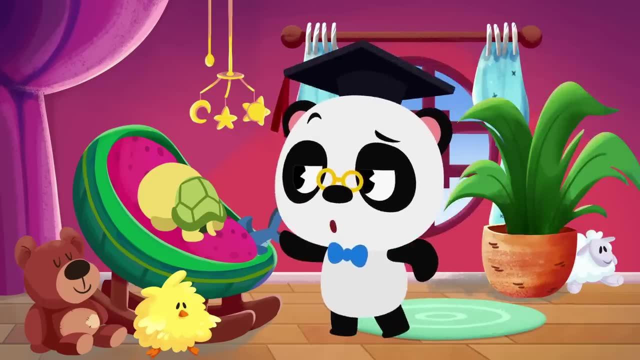 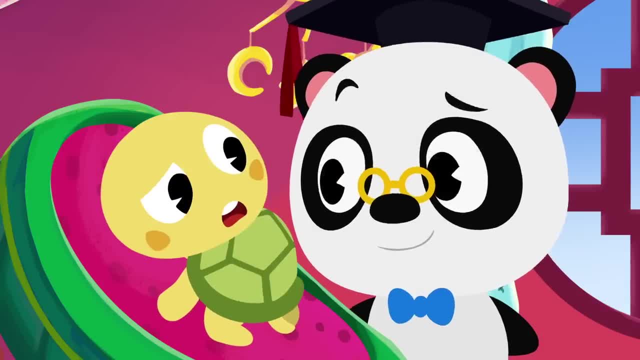 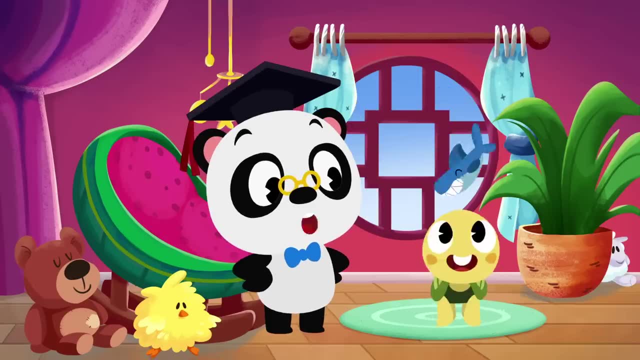 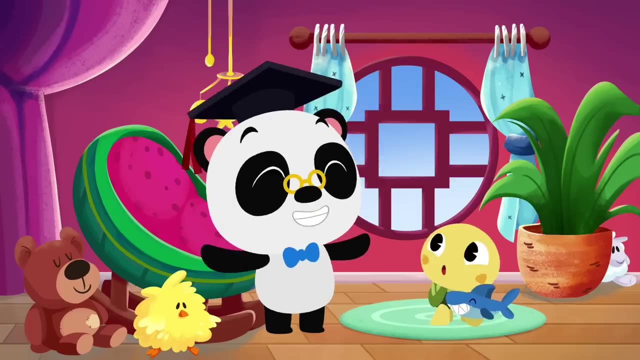 and has sharp teeth. Huh Ta-da, I found your toy shark. Yay, Come on, Toto, We can finally go to the supermarket. I'll buy you and your shark some ice cream. Yay, Hi everyone. 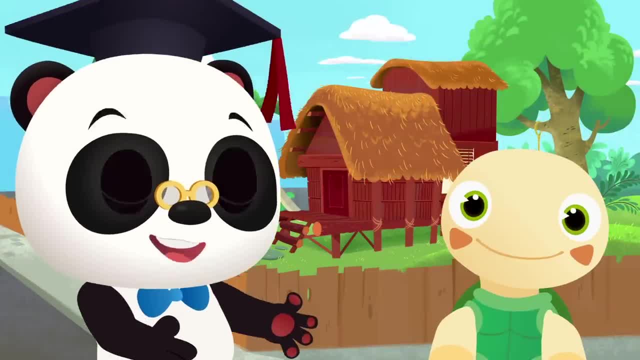 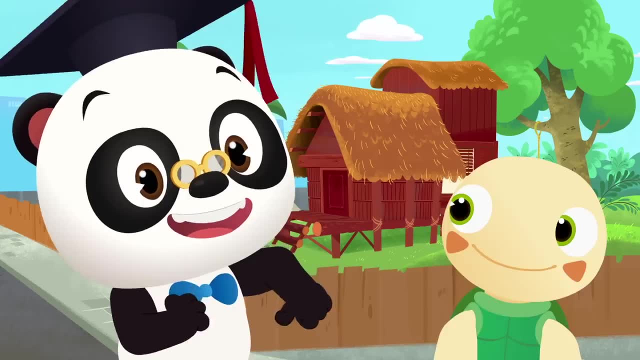 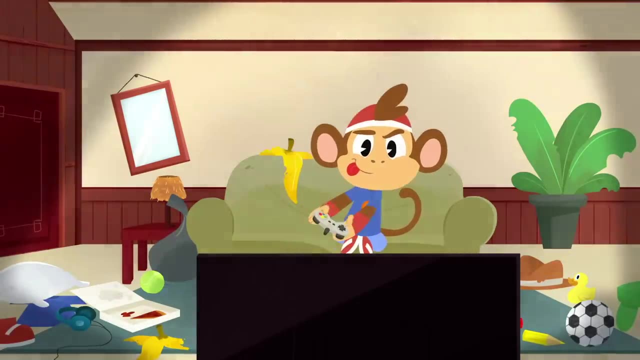 It's Dr Panda Toto time. Today we're visiting Bip's house. Bip, Bip, Let's go and see what Bip is up to today. Yay, Hey there, Bip, Have you got plans to go anywhere or see anyone today? 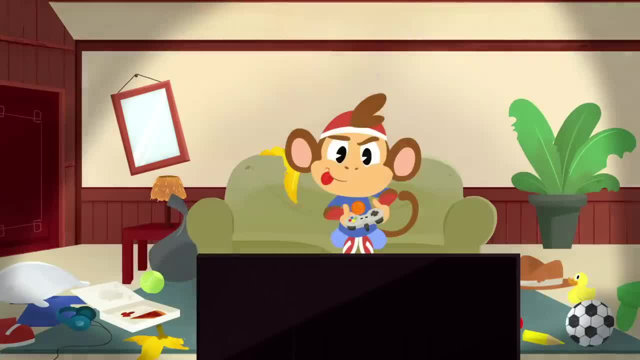 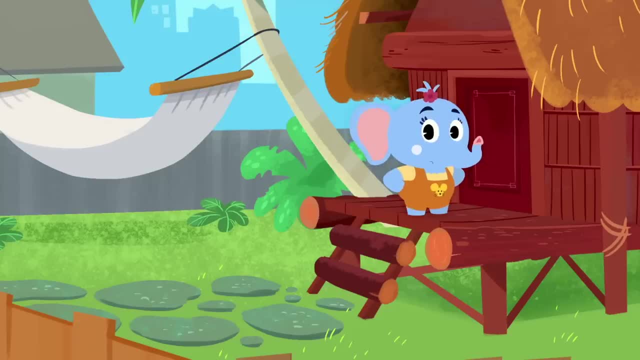 Hmm, looks like Bip's pretty caught up in that game. Aren't you going to answer the door, Bip? Oh, it's Ouellette. Hi Ouellette, I thought you'd be practicing for your basketball game tomorrow. Oh, I get it. 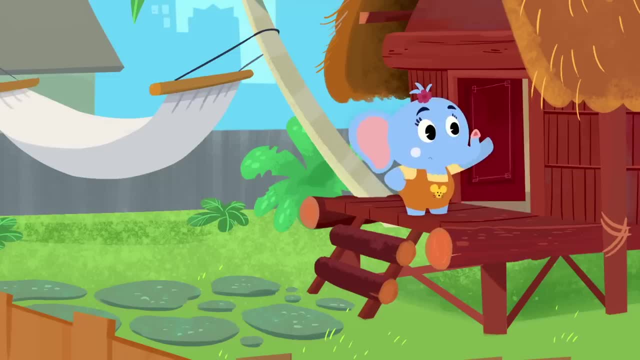 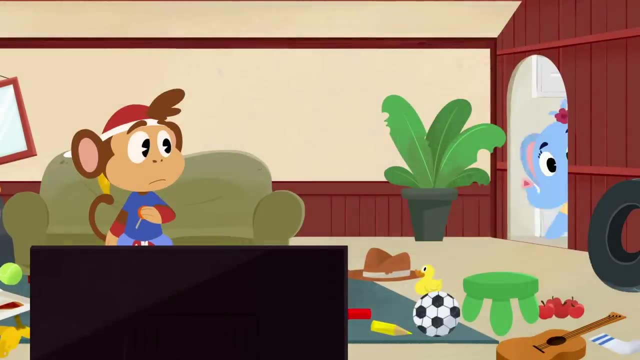 You lent your basketball to Bip. Oh, look, It's already open, Are you all right, Ouellette? Uh, Bip, Ouellette just had an accident because your house is so untidy, And how are you going to find her basketball? 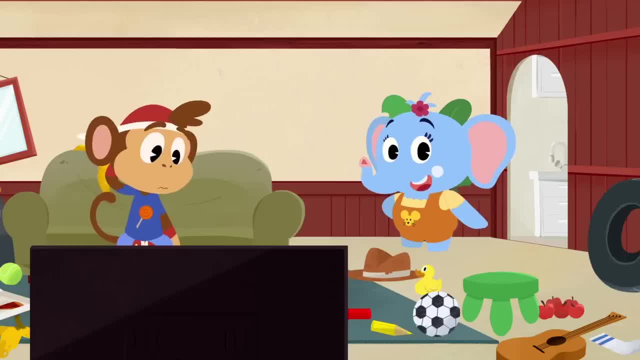 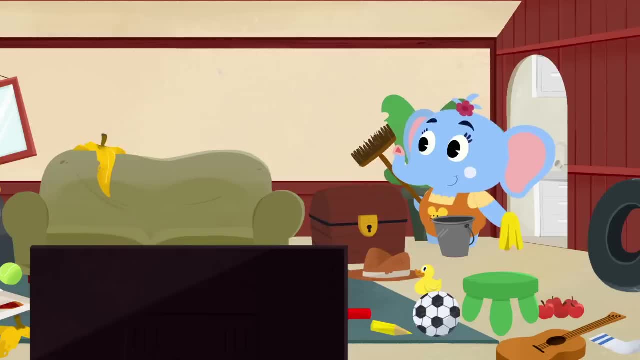 in all this mess. Are you thinking what I'm thinking, Ouellette? It's time for a big spring clean. Don't worry, Bip, We'll make it fun. Let's start with tidying away the toys in your living room. 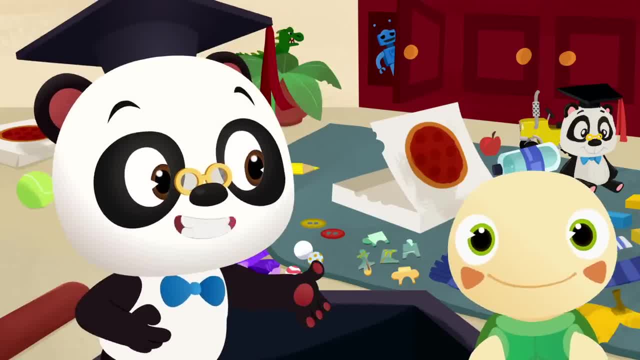 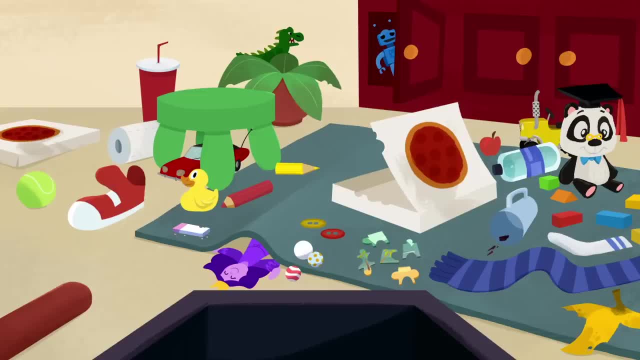 Can you help Bip find the toys that belong in his toy chest? Can you see his red racing car? Great. Now can you spot the green dinosaur- Good job. Do you see the blue robot? Awesome Now can you spot the yellow tractor. 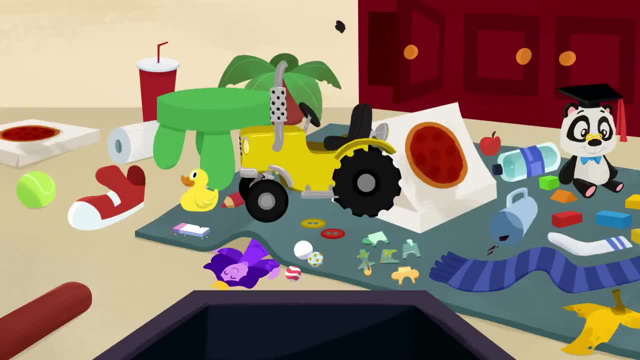 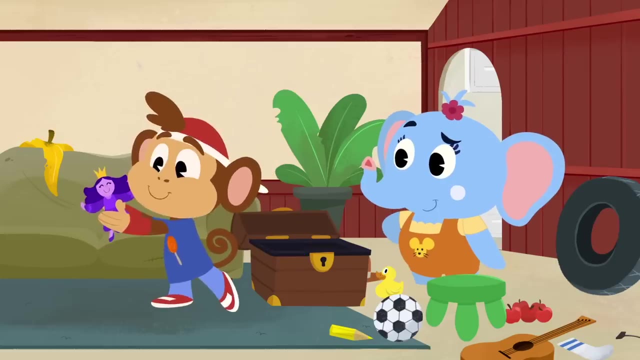 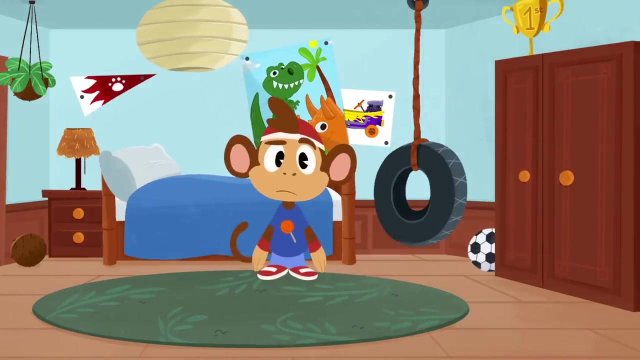 Good job. Only one more toy to put away now. Can you find the purple princess? Great job guys. Now all Bip's toys are tidied away. Hi Bip, Have you found Ouellette's basketball yet? Hmm, Have you checked the closet? 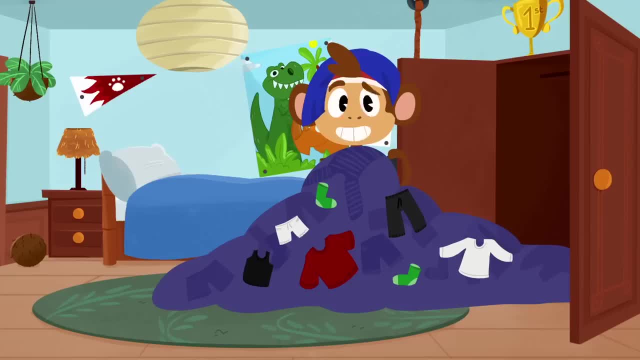 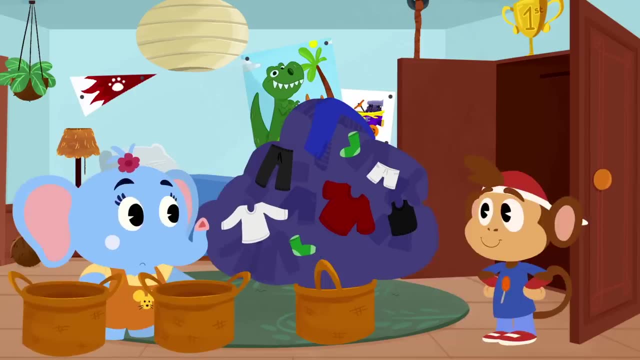 Whoa Uh, Bip, Bip, Bip. I think it's time to do some laundry. That's right, Ouellette. You can't put all the dirty laundry together. You need to separate the white, the colors and the dark clothes. 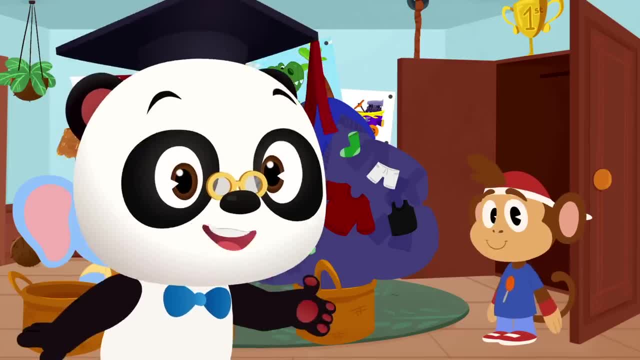 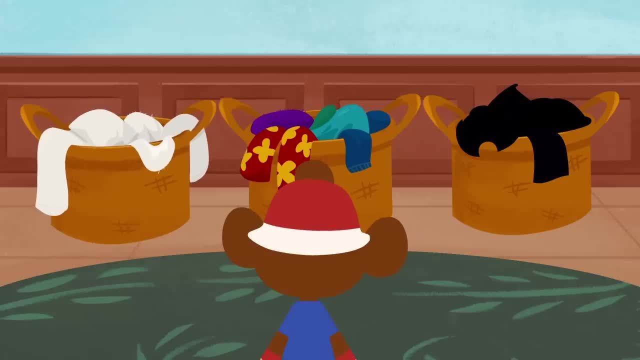 Maybe you can help Bip separate his dirty laundry. So the white clothes go in the basket on the left, The colors go in the basket in the middle And the dark clothes go in the middle And the dark clothes go in the basket on the right. 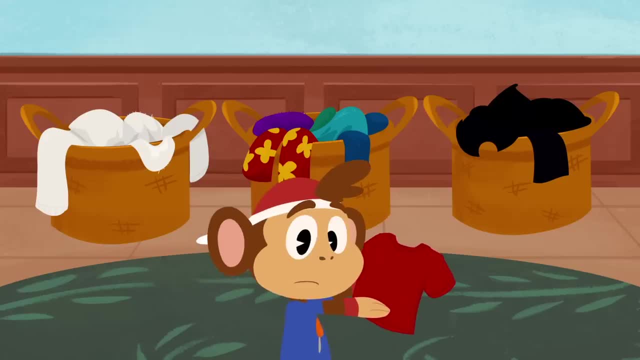 Is that shirt white, dark or a color? Color, Color. That's right, It's a color. So which basket should Bip put it in? It goes into the middle basket Score: Yay, Where does this go? It goes in the dark pile. 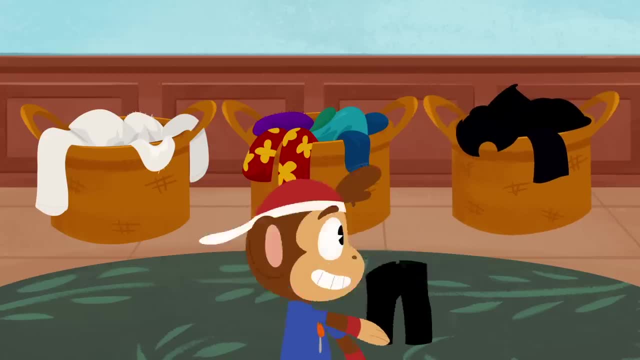 Shoot for the basket on the right, Bip. Oh, hang on, Bip. Have you checked the pockets? Score Wow. And where did these go? They go in the white pile. Aim for the basket on the left, Bip- Awesome. 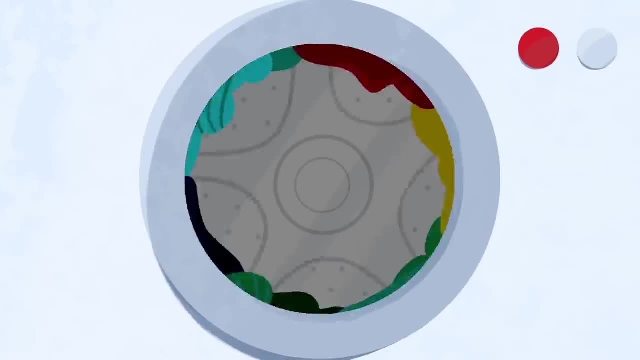 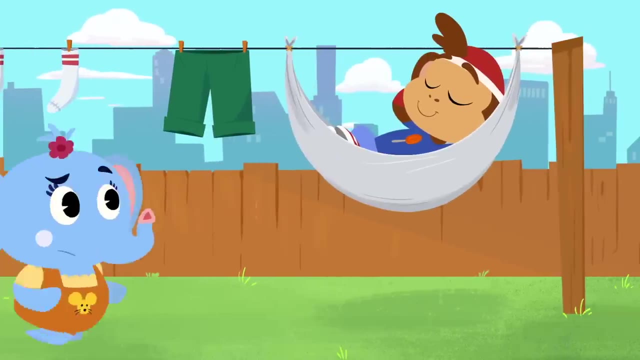 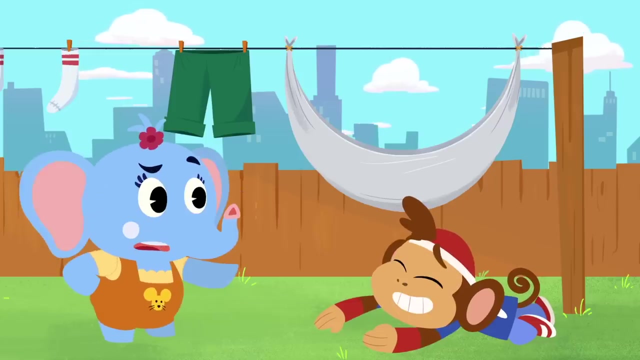 Now let's go wash the laundry. Bip's threw in your one Up, you get Bip. There's still lots of other things to clean while you wait for your laundry to dry and you still haven't found Olette's basketball. Hi Olette. 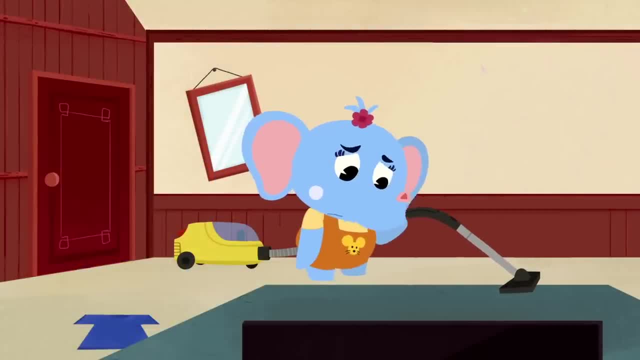 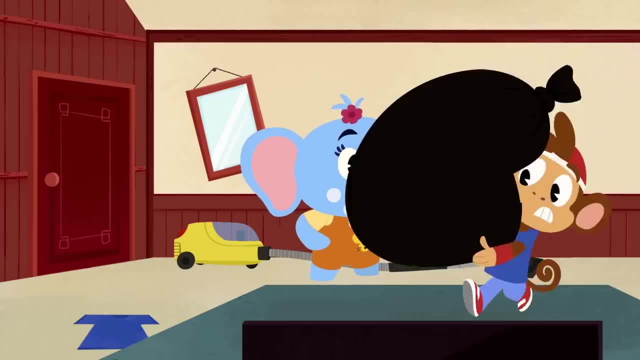 Have you found your basketball yet? Not to worry, If you and Bip keep cleaning up the house, it's sure to show up somewhere. Whoa there, Bip. That is wonderful. Let's go. Let's get you out of here. 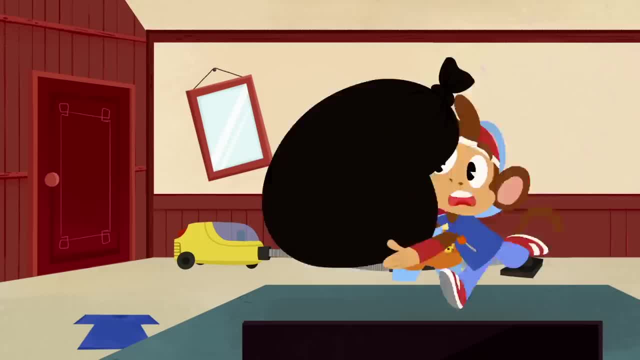 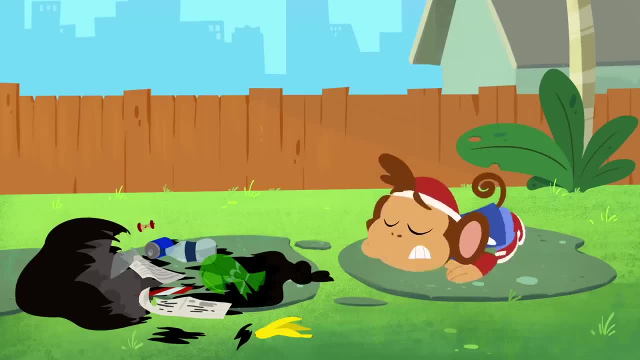 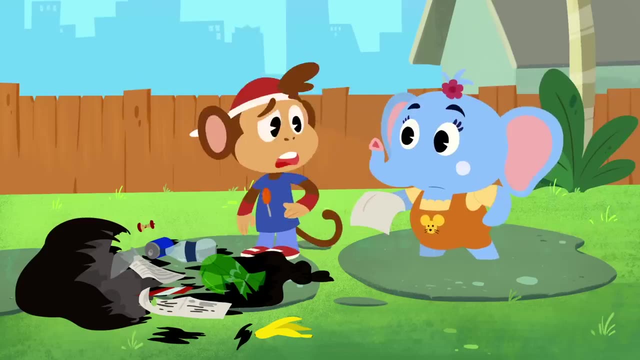 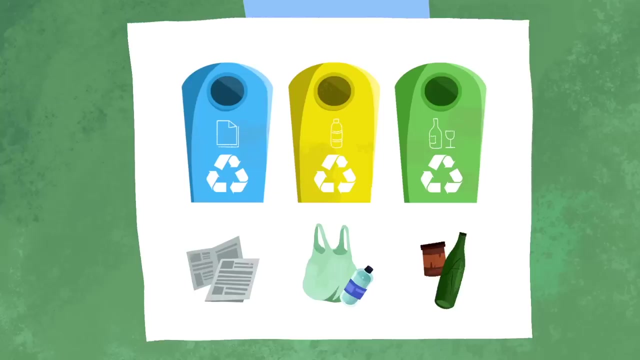 Okay, We must be late. That is one big garbage bag. Watch out, Uh-oh. Are you okay, Bip? You'd better pick up all that garbage before it blows away. What's that, Olette? Oh look, This shows you how to recycle all your trash, Awesome. 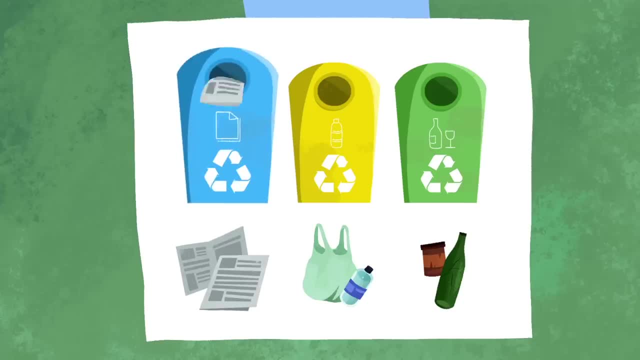 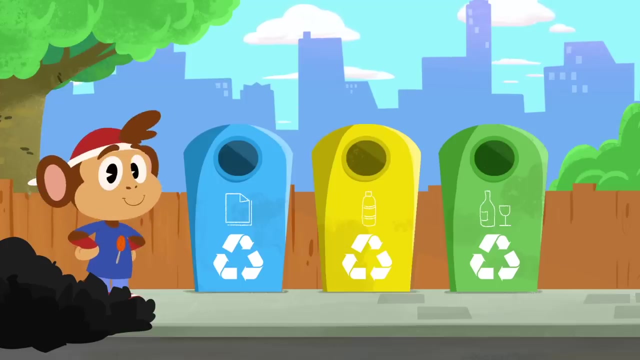 So paper goes in the blue bin, plastic goes in the yellow bin and glass goes in the green bin. Hey Bip, Time for a new game. Let's pick up your trash. and figure out which bin it should go in. Can you help Bip remember which bin he should use? 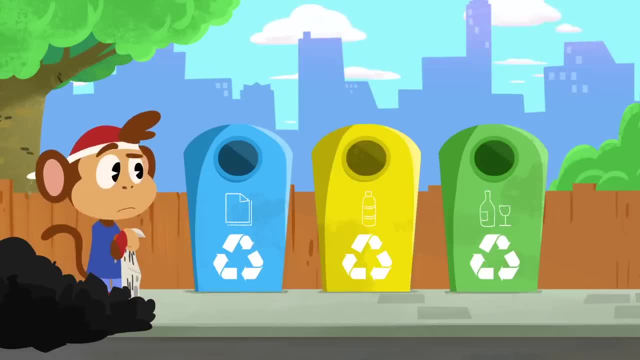 An old newspaper. Okay, let's see which bin does paper go in? That's right. The blue bin is the bin for paper. Let's see what's this bottle made of. Is it plastic Or glass? That's definitely a plastic bottle. 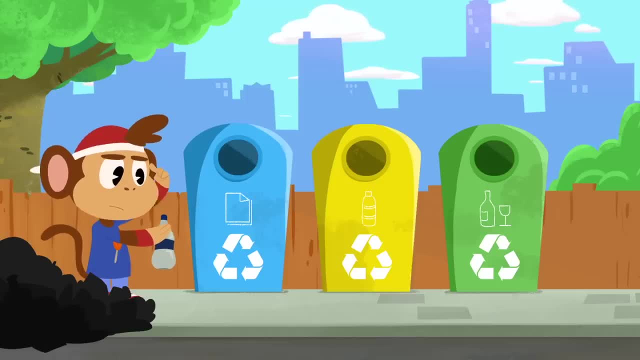 So which bin does the plastic go into? Yep, you got it. The yellow bin is for plastic. Careful with that one Bip. You don't want to play around with broken glass. It could be very sharp. Now, which bin was for glass? 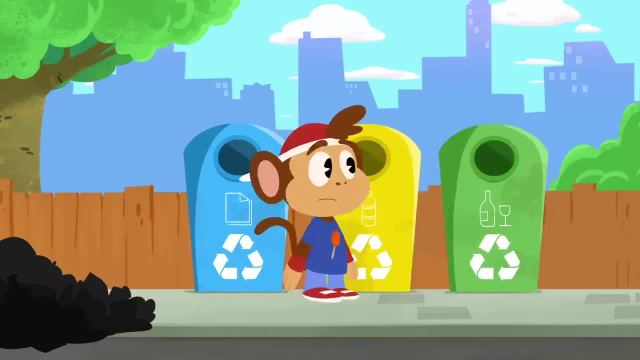 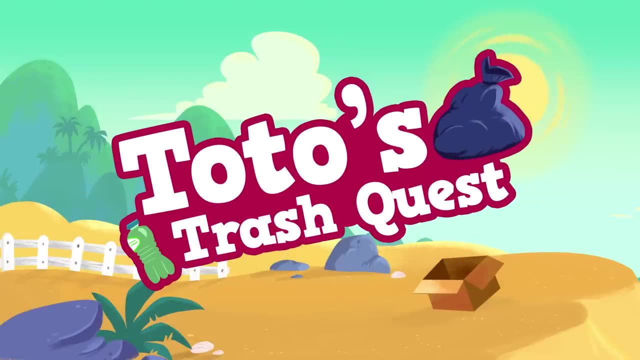 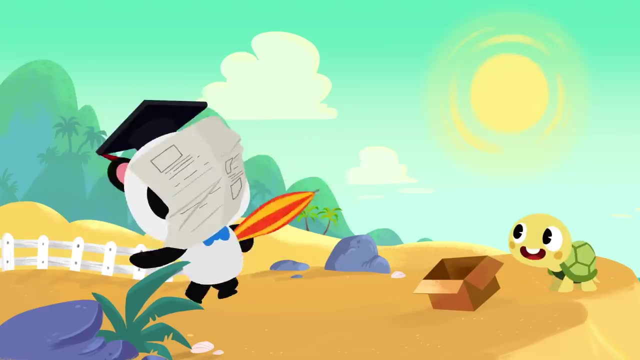 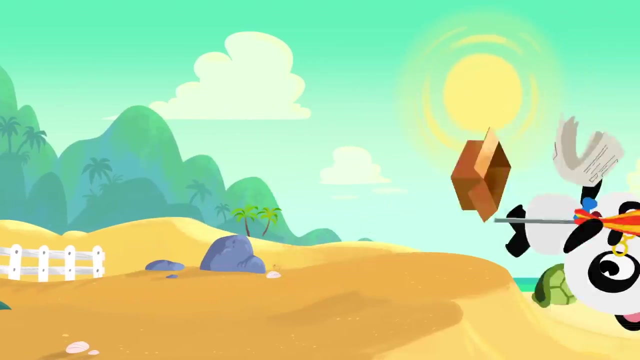 Yep, The green bin, That's the one for glass. Now all your garbage is in the right bins. Awesome job. Ah, Toto, It sure is a lovely day for the. Oh, as I was saying, it sure is a lovely day for the b-b-b-beach. 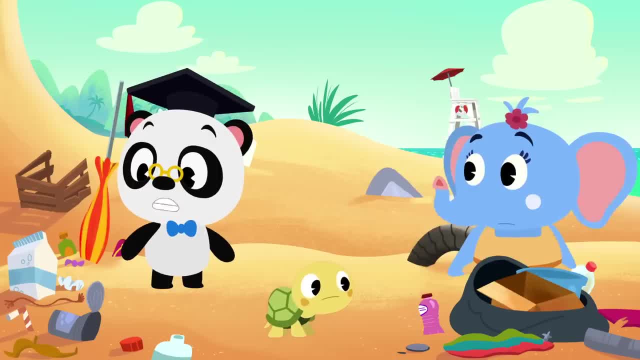 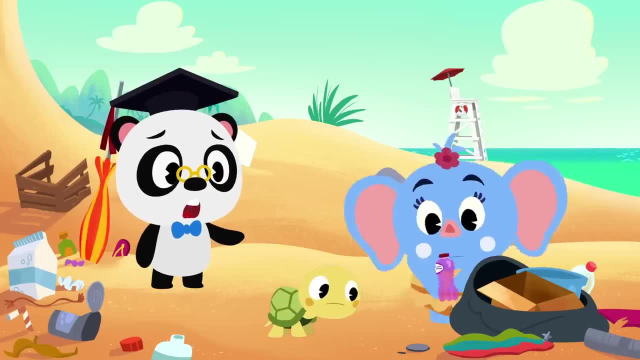 Thanks, Olette. What's all this trash doing on the beach? There's not even a clear spot for us to put down our beach towels. Will you be able to clean it all up by yourself, Olette? No worries, Olette. 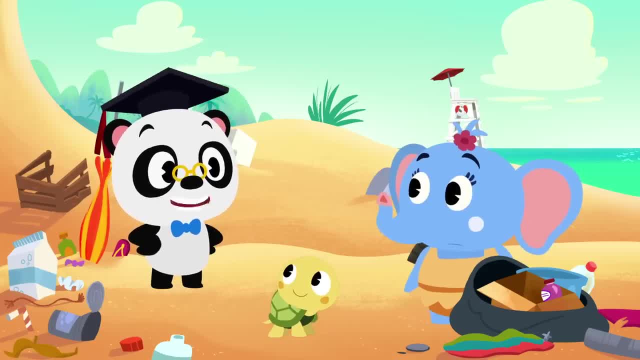 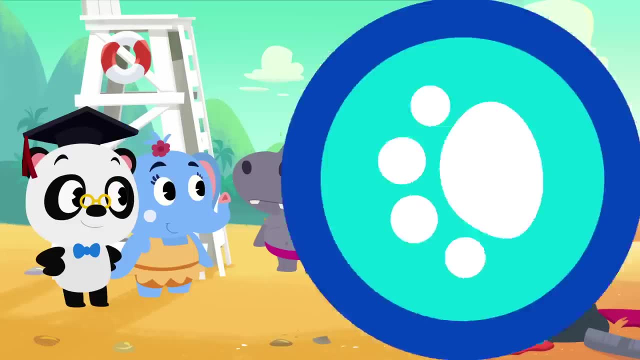 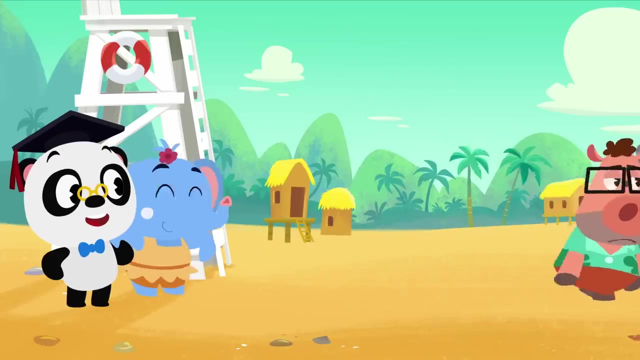 Let's call our friends and ask them to help. If we make a game of it, we'll have the beach cleaned up in no time. Yay, Game, Alright, guys. Whoever fills up the most trash bags wins the game. Let's see. 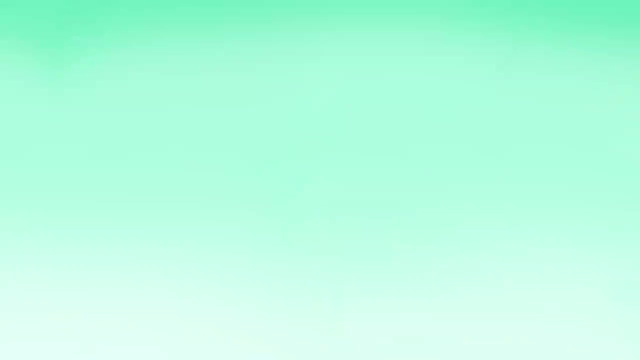 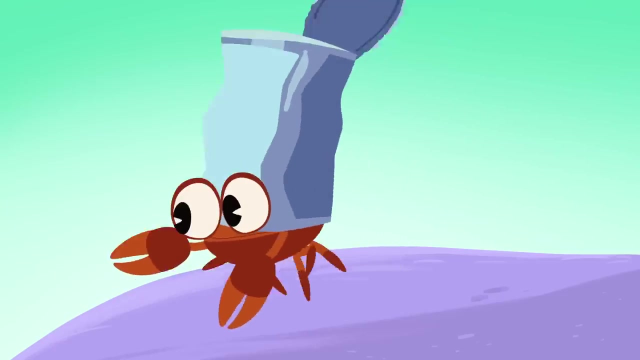 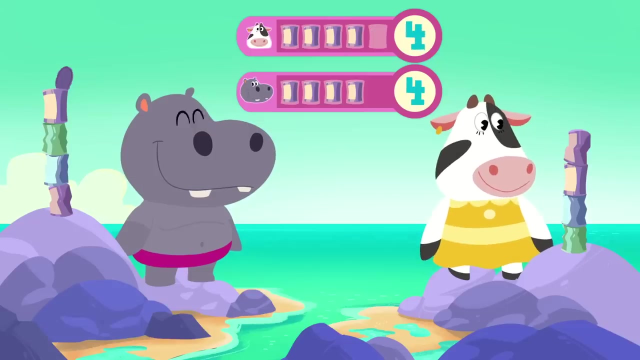 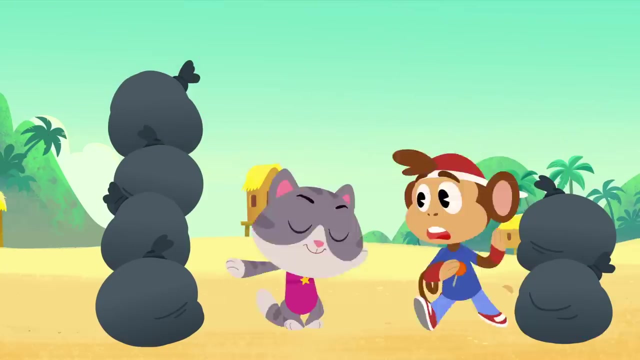 Poopa has collected four cans And Moo has collected five cans. Uh-oh, That last can was that little crab's house. Now Moo only has four cans. Poopa and Moo have the same number of cans. Nice work, Maymay. 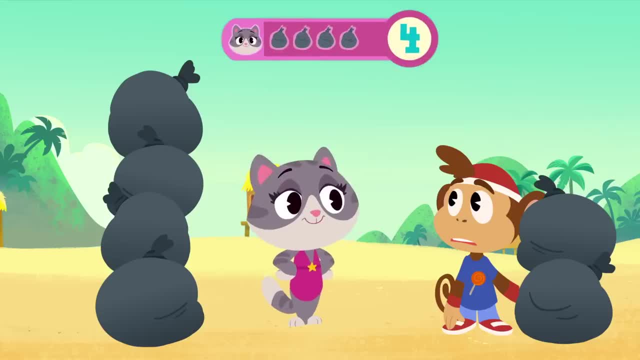 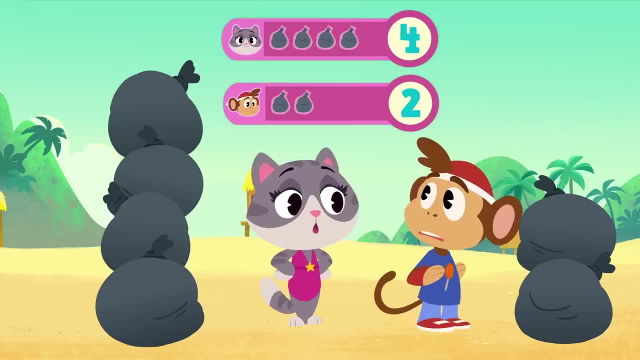 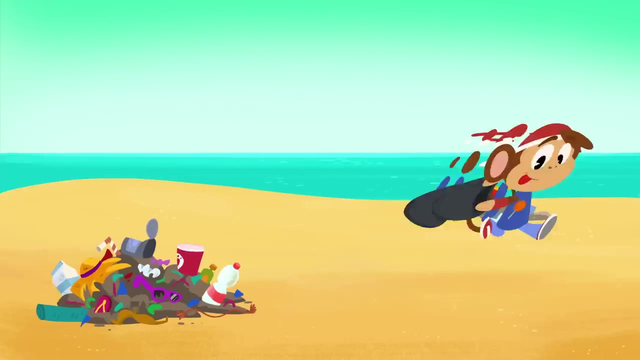 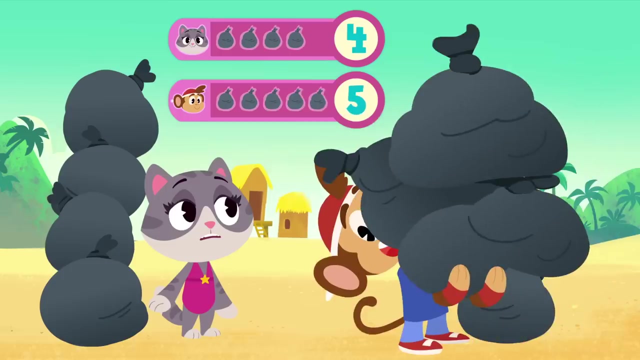 You've already filled four trash bags. You filled two bags Bip. That's fewer bags than Maymay. Better get to it if you want to win this game. Whoa Bip, That's awesome. You have five bags Now. Maymay has fewer bags than Bip. 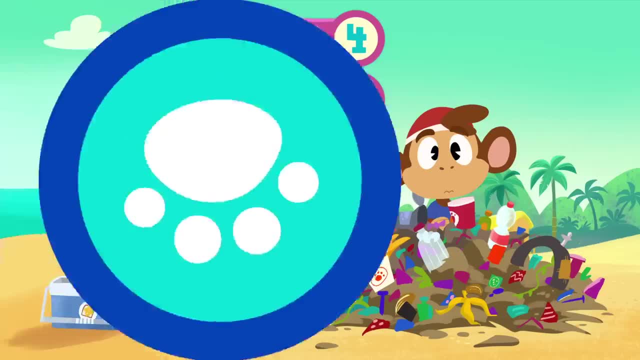 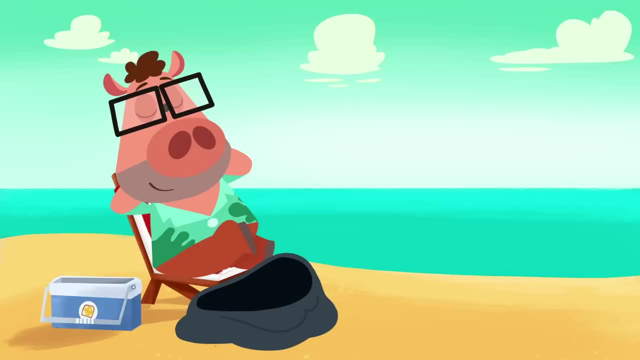 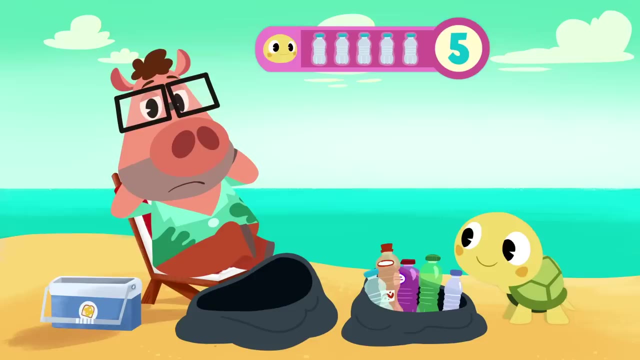 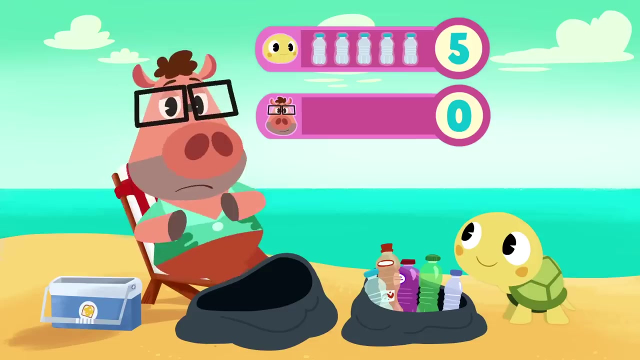 Haste makes waste Bip Better. start over Awesome work, Toto. Toto has collected five bottles, Yeah, And Ziggy has zero bottles. That means Toto has more bottles than Ziggy. Come on, Ziggy, You can do better than that. 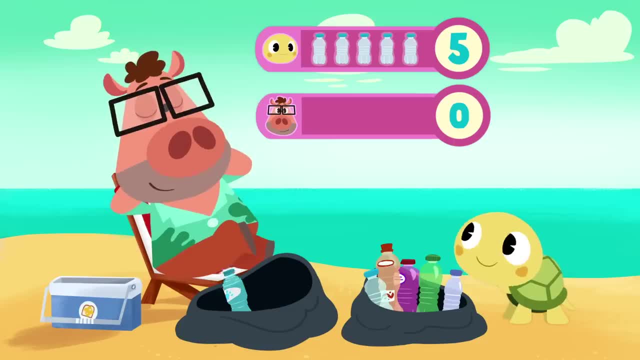 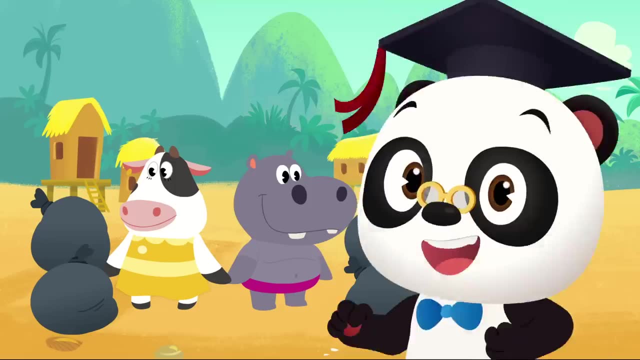 Well, I suppose that counts. Now you have one bottle. One bottle in your trash bag. Thanks for putting it in the bag and not throwing it in the ocean. All right, Let's see who has filled up the most bags with trash. 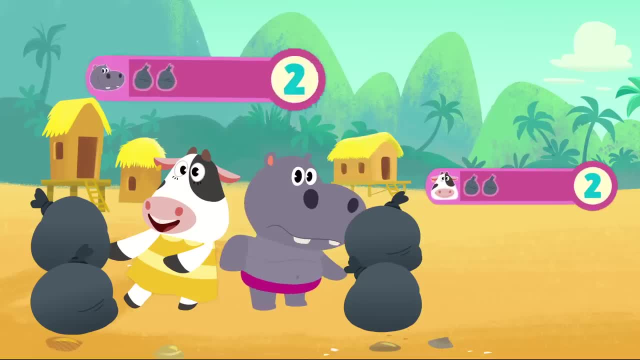 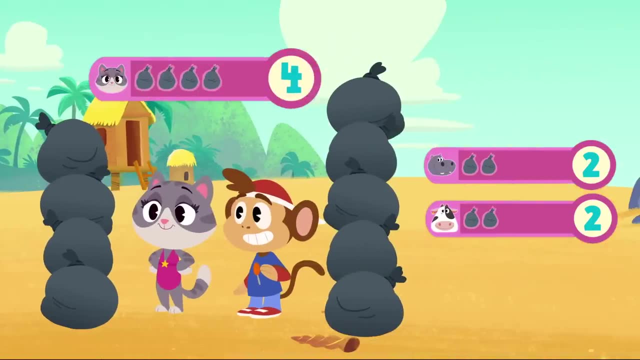 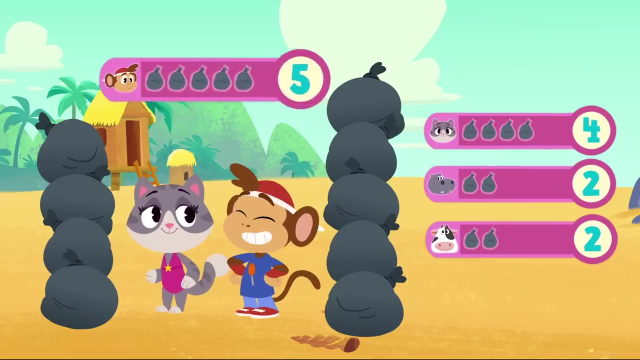 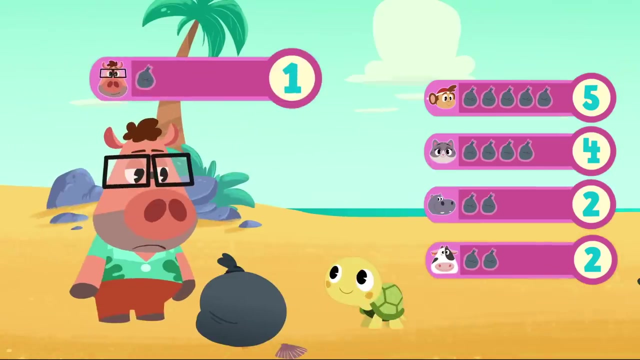 Moo has two bags And Poopa has two bags. They have the same number of bags. Maymay has four bags, which is more than Moo or Hoopa, But Bip has collected five bags. That's more than Maymay. Ziggy has only got one bag of trash, which means he has collected less than everyone else.